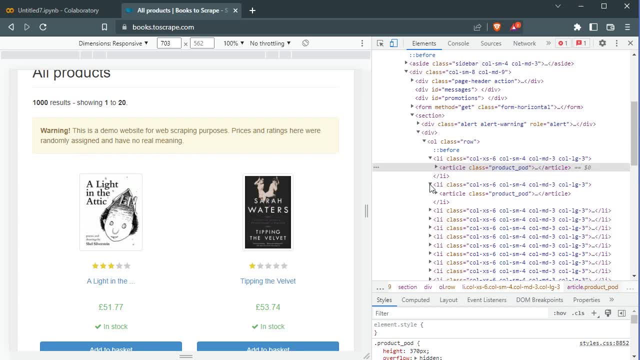 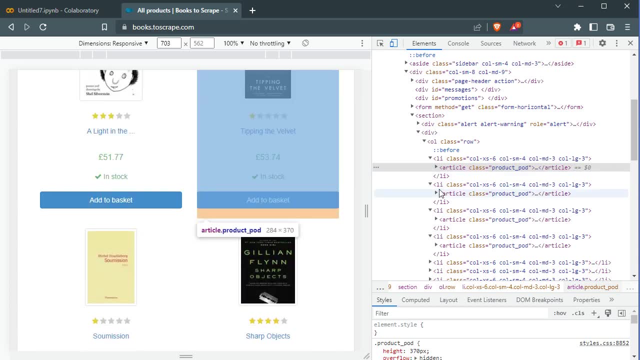 If I go over this one, you see, this one is highlighted, you see. And then for the next one, you see, this is highlighted. And lets say, let me open some of them. If I go over this one, you see, this is highlighted and this one is highlighted. 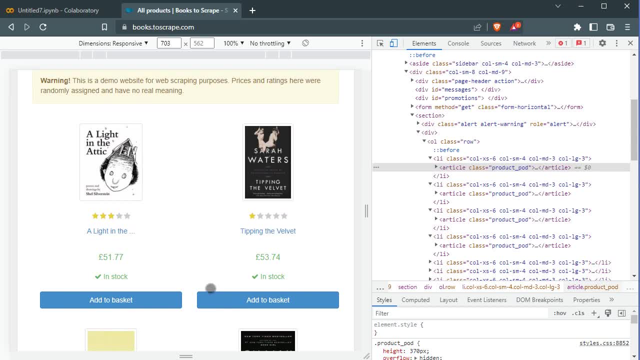 So all of these cards, these are cards which are included in a list item, inside an article tag With the class of product: underscore: pod, score, pod. so if I want to get access to the title of this, to the stars and to the prices, I need to target or send a request to get this page and then target. 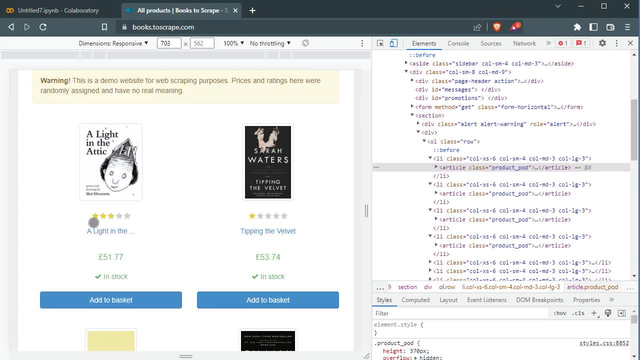 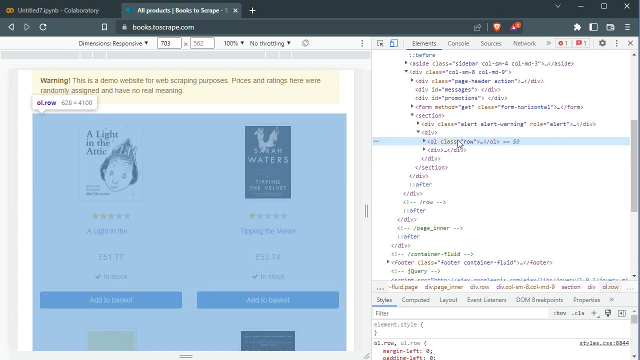 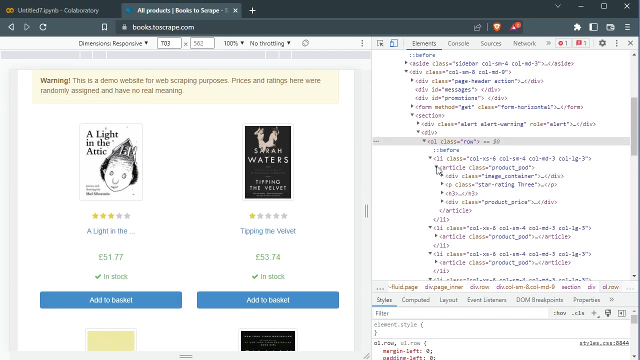 the tag which is responsible for displaying this information and in our case it is the article tag. inside the unordered list you can see when I hover over it all of it gets highlighted. it means everything we needs inside this ordered list, Oh, L, and then you can see article. if I expand article, you see we 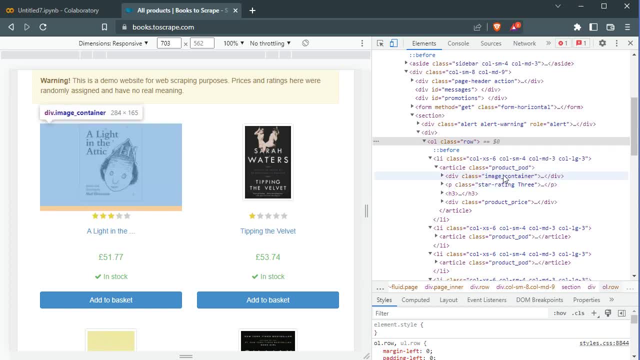 have a map image container and this gets highlighted by hover over it. there is a star rating and you can see there is a h3 tag which has the title in it- well, parts of the title, because it's a bit long- and then we have a product price, which this part is all about, and you can see. 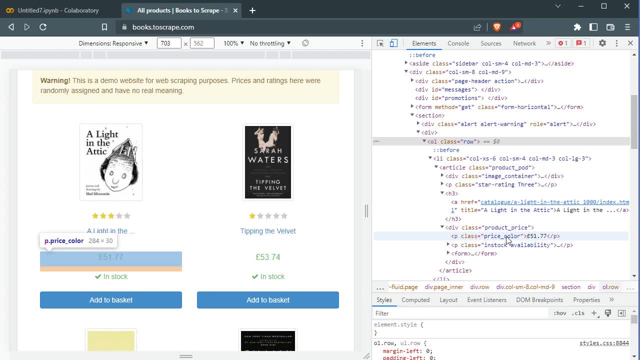 here under a paragraph tag with the class of price color. I can find it okay. now the issue is: if I go under title, I can't see the full title here. so where can I get a full title of this book? well, I have realized that under this image. 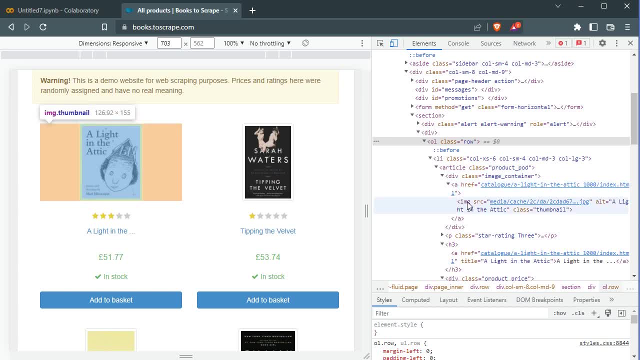 container, inside this, a tag. there is a tag and it has an alt attribute which is more like a description of the image and you can see this alt attribute has the full title. so we are going to get the value of this alt title and put it inside the titles of our books. the same: 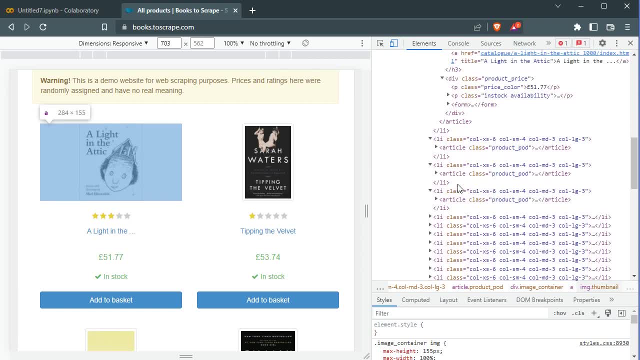 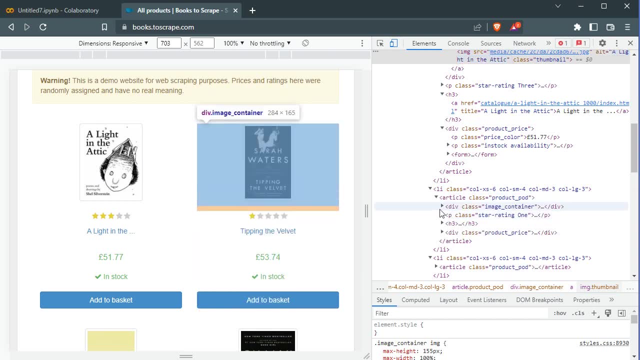 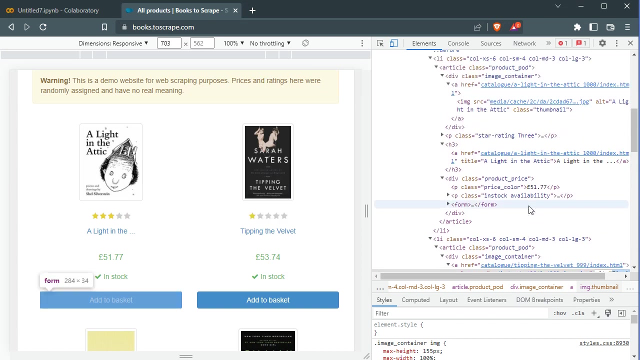 is true for the next one, the same exact process. so if I go to the second list item, an article you can see on under image container and under the a tag there's an image, and this image has an alt of tipping the velvet, which is the name of this book. you can see again the stars as well. now, what about the stars? 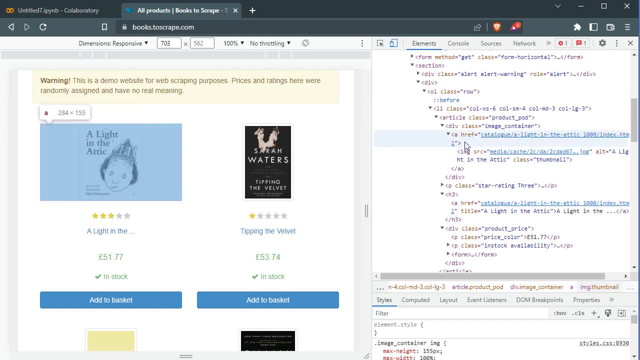 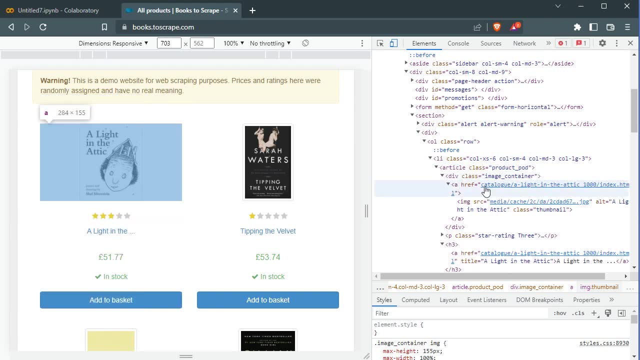 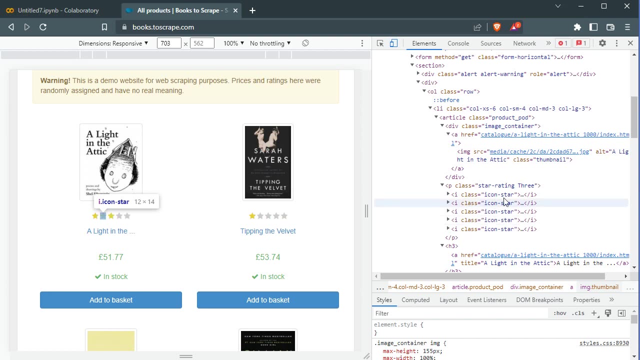 how do I get the number of stars? it's interesting that inside this article tag- the article tag here- so we had the image- we had now the star rating- you can't find any useful information here. the useful one is this: class name three. so this three, which is the name of a class of this paragraph tag, refers to. 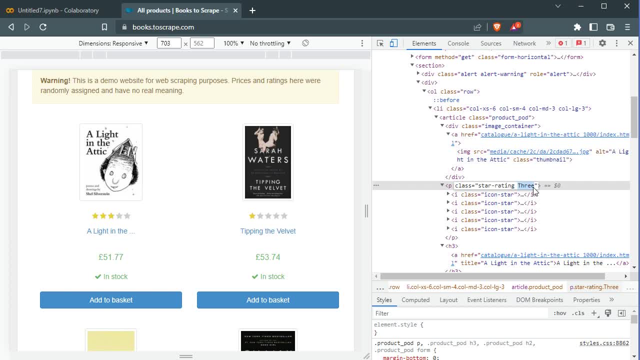 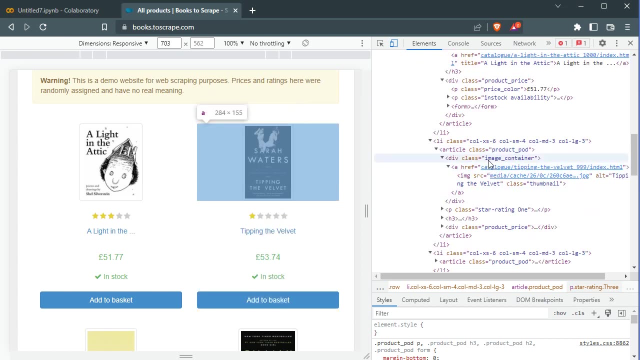 the number of stars it has. so what we can do is to grab the name of the class of this paragraph tag and put it as a star rating. so, for example, this book tipping the velvet has one star. if we go down below and under star you see P class, star rating one. so it has only one. 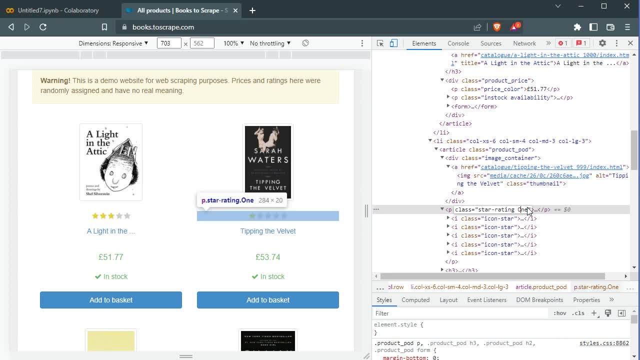 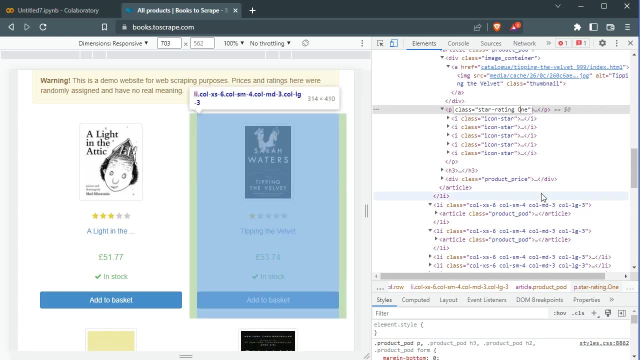 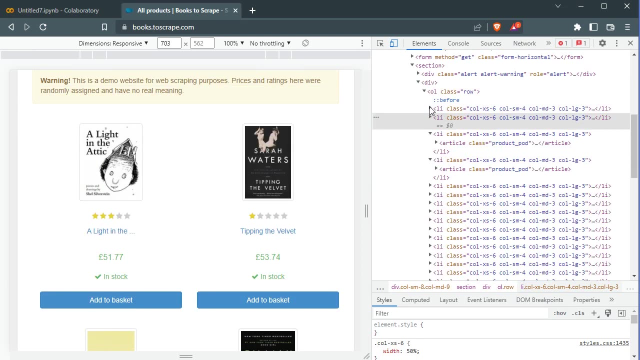 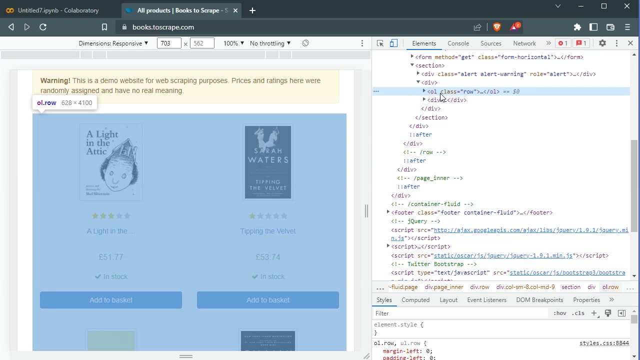 star. that is how we are going to grab this star rating, and you also saw how we do it with with the price tag. okay, so again, the last time, what we need to do is to have access to this page. then we need to go into this, or l grab this whole list and we'll loop. 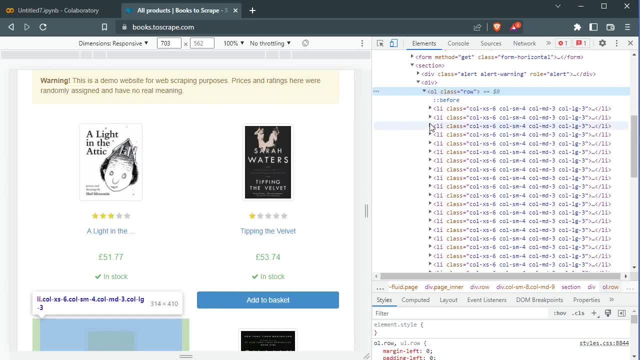 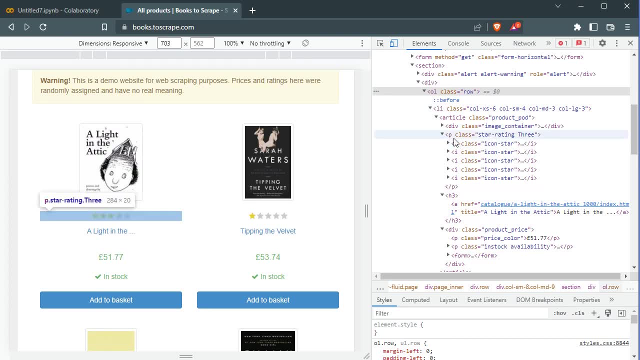 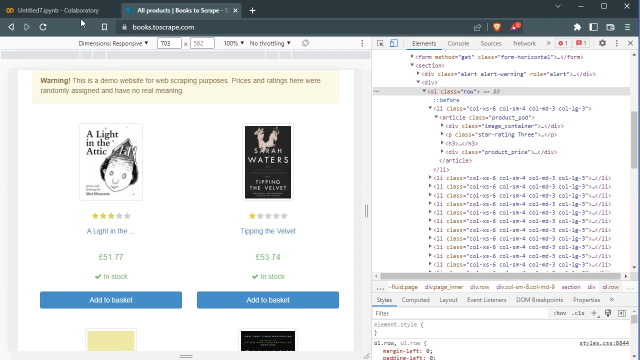 through each item to find the article and then inside every article we are going to find the images, ult, the star rating and the price of that article, and then we семь lik vulcan. now let's get to coding. so I'm opening, I've opened this colab of Google, so this: 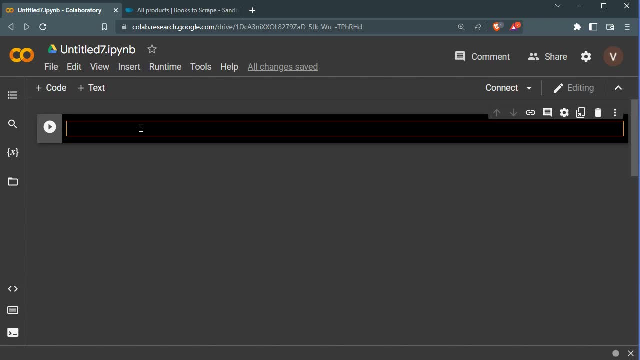 is an online IDE, that is, I don't need to install any libraries on my own machine. I do it here. the first thing we need to import is the requests library, and if I press shift enter, it goes to the next cell. it runs it as well. now I have. 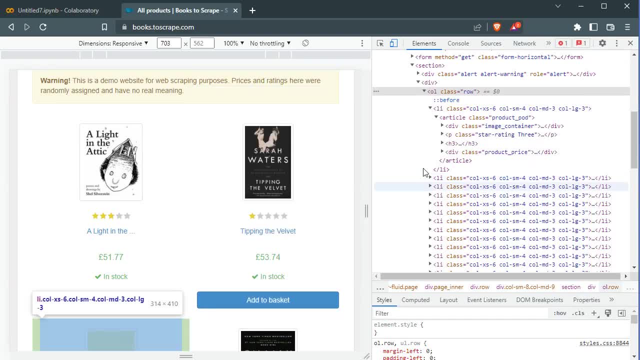 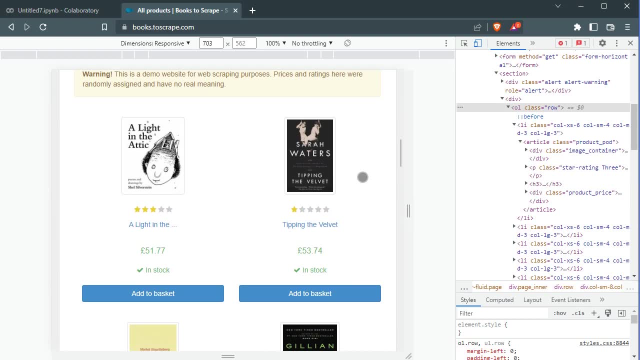 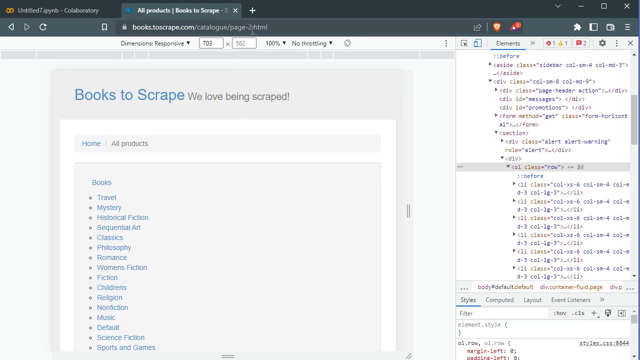 access to this library so I can send requests to grab this web page. and now let me see how. so if I go down below, let's say press next, for instance, and you can see we have page 2. I want to go back to page 1 and I will tell you why. 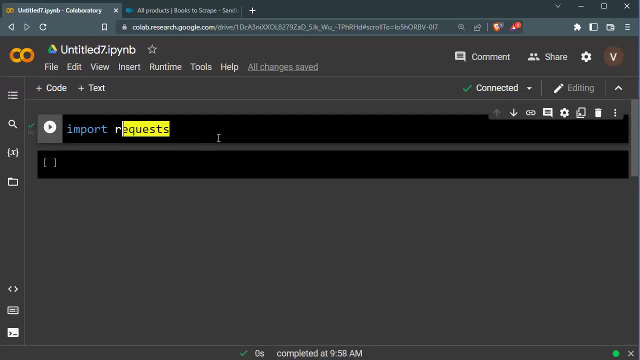 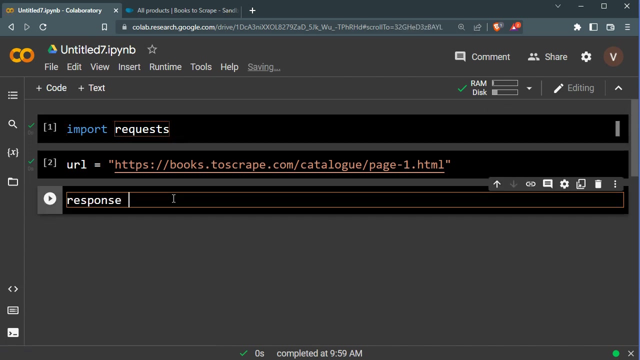 I've done that one, okay. so I am going to copy this URL and put it inside a URL variable and inside double quotes. now I'm going to send a request to grab some response from this. so I'm going to say: response equals requests dot get. so I'm going to 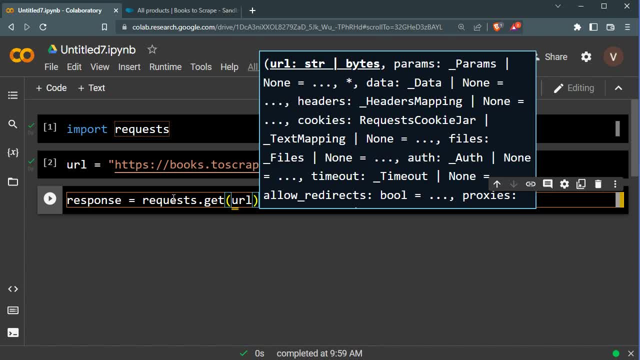 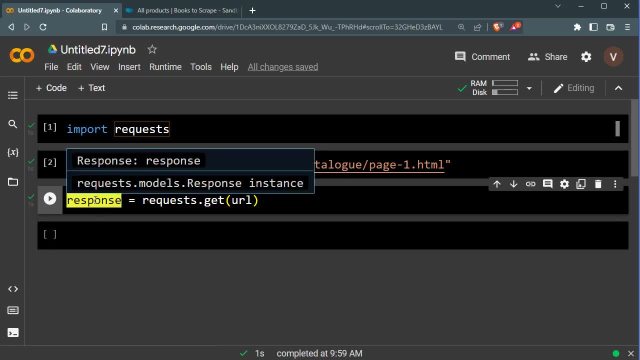 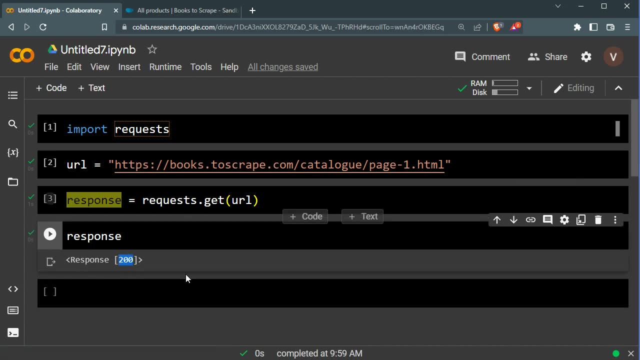 send request to get the URL. so if I run this I don't get anything here now. but if I print response, if I print response here, you would see I get a code of 200. it means this request response was successful. so we have access now if we got something. 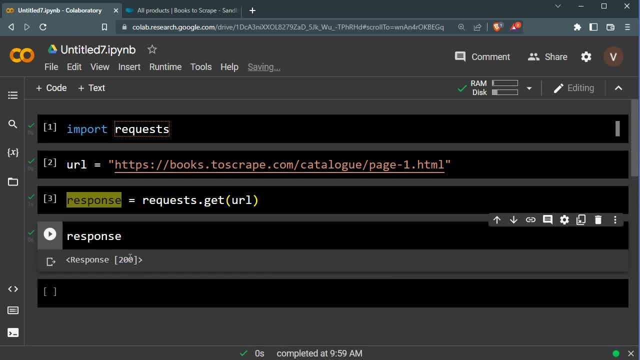 like 404, it means the page was not found. so there's a list of all these codes- response codes you can find online. now I don't need this code, it's not that useful, so what I need is actually the contents of that response. so that's why I'm going to save. 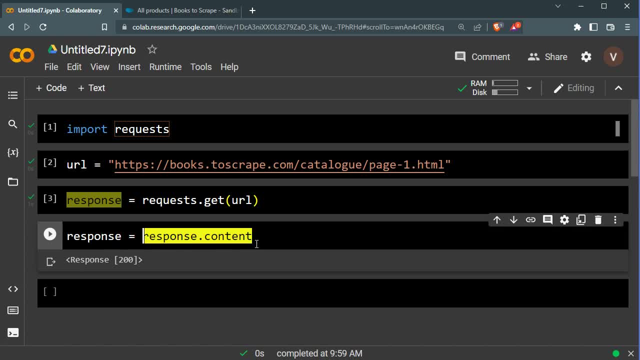 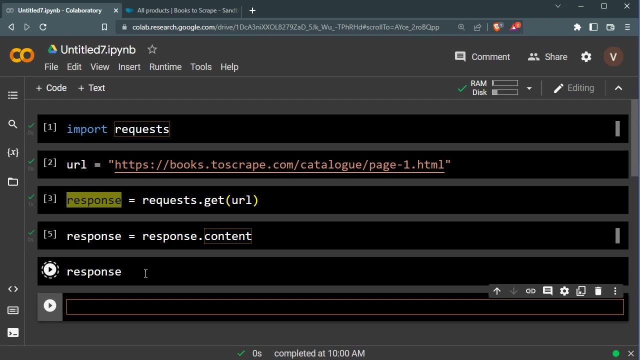 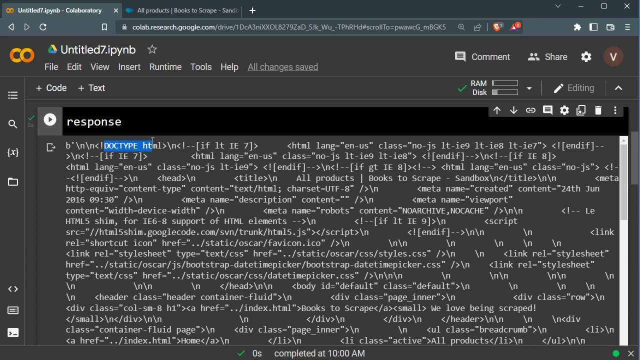 the responsive content into response now and run and run this now. if I run response, you would see a huge binary. it's like a like a string kind of, and you see all this. the HTML code is in here, but this is not HTML file. actually, you can see this be here, so I need to turn this into HTML code and get access now. 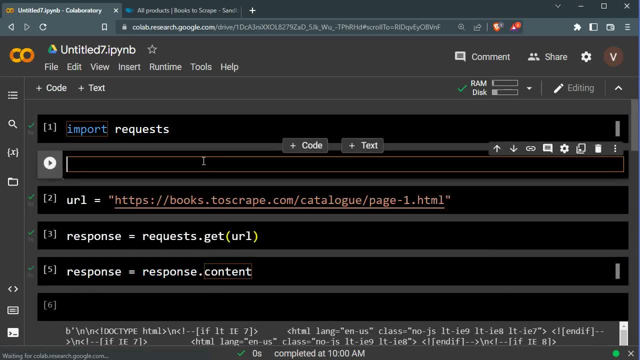 this is where soup comes in. so we are going to import from, well, from bs4, import beautiful soup. let's see. if it suggests yeah, and you can see uppercase B, uppercase s. so beautiful soup is going to be the library. let's run this. we are going to. 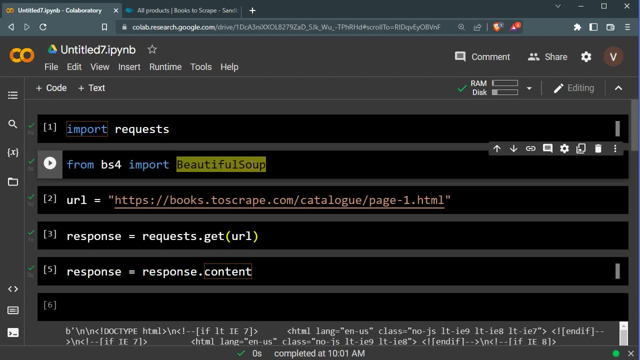 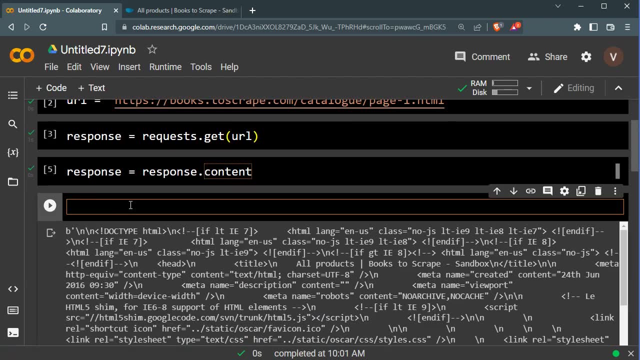 use to scrape the website. the first thing you need to do is let's copy this down here, the response that we got right. we're going to make a soup variable- you can call it whatever you want, though, and we are going to use a beautiful soup class that we just beautiful so that we just received, and we are going to pass. 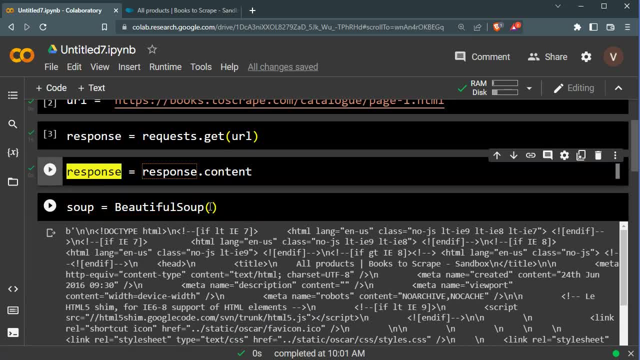 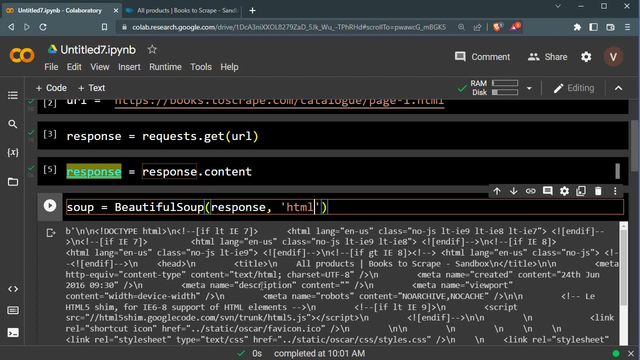 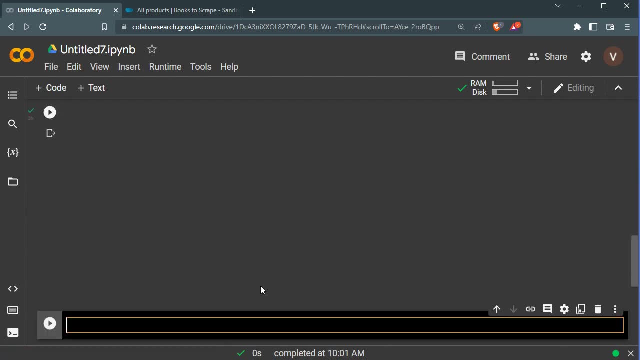 in two arguments. the first one is the response that we just got and you see it. see here this one. but we need to specify: this is an HTML page, so we need an HTML dot parser to parse this HTML for us. now I run this and if I run soup, to see what soup is, 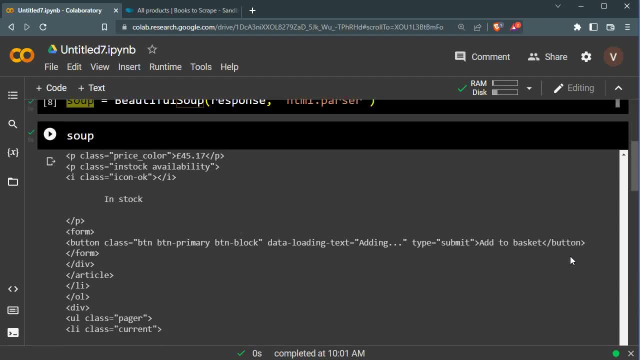 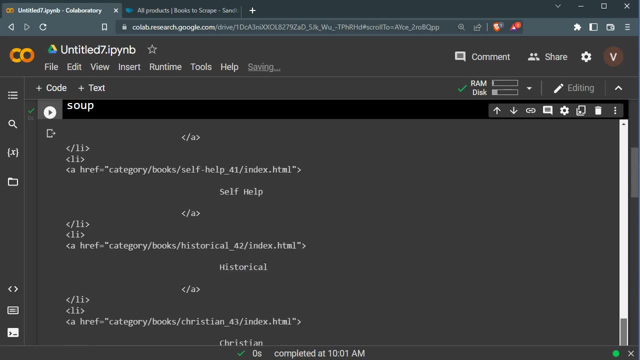 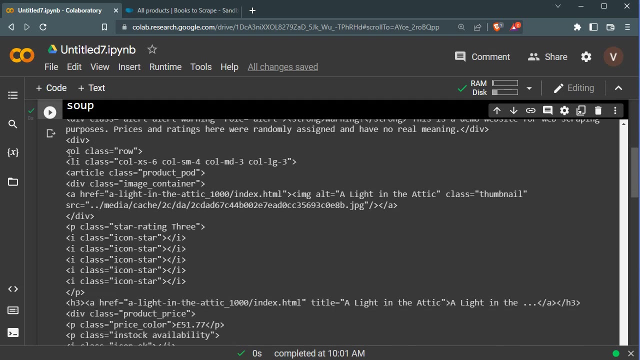 now, soup is the HTML code. you can see it here now. so HTML code, you see the list items and all that. so if I go down further below under section section, let me see. so there, this is the order list we are going to grab, which contains all the lists and articles. you see, inside article we have this. where is the? 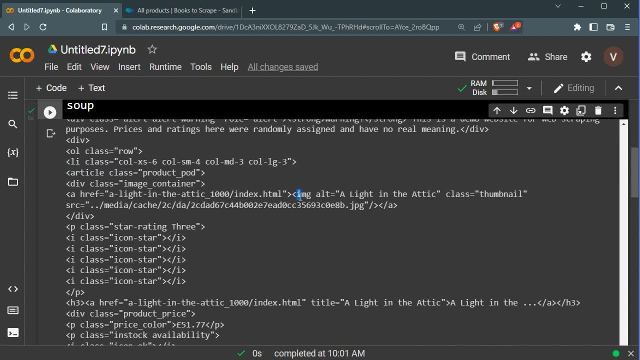 image, this image. you see this image and the alt attribute. this is the name of the book. then if we go here for a star, under P tag there is a class of three, which means it's received three stars. and then for the price. so we have it here again, a P tag with a class of price color. 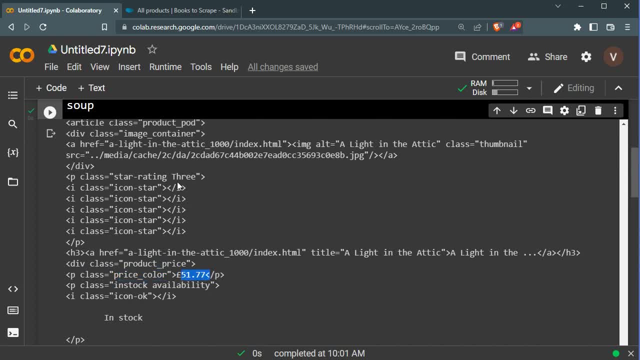 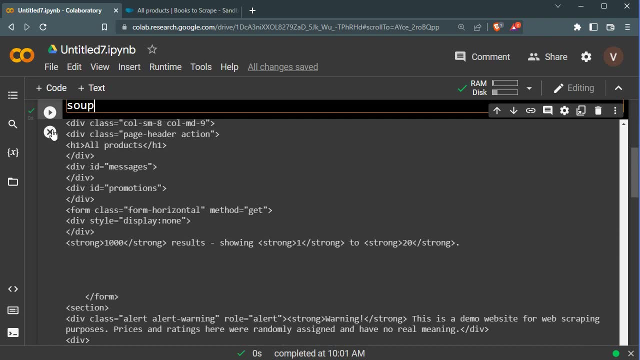 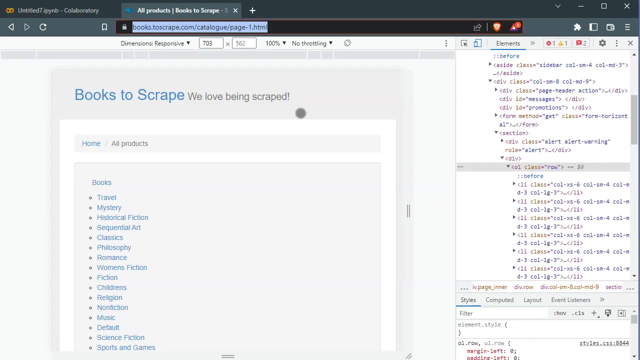 and this is the price. so we need only three, these three pieces of information. okay, so this is soup now, as you just saw. so I said we need to grab the order list within that soup, right? which is, or was that ordered list? yeah, here. so we need to grab this order list because all the 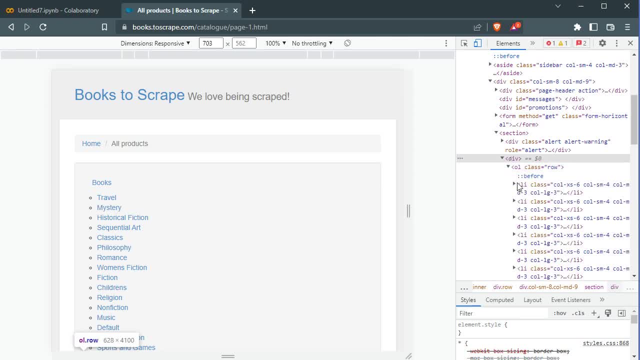 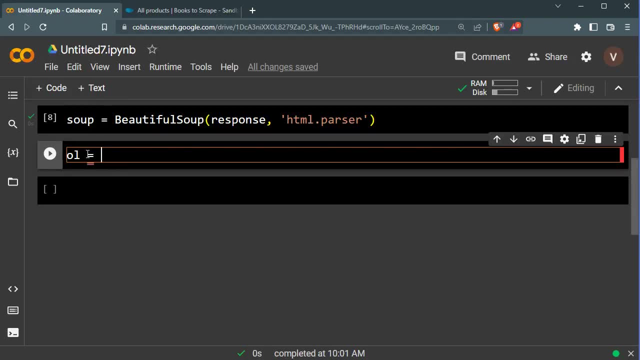 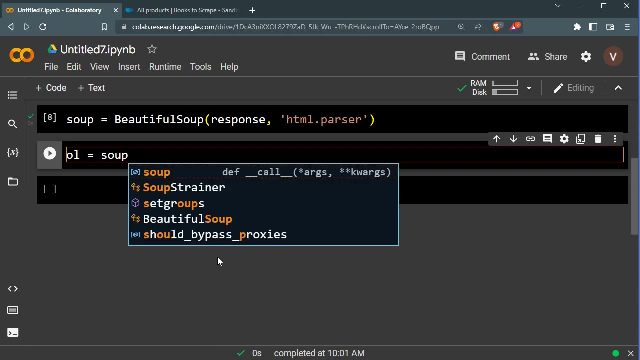 cards. all the books are within the lists. inside is order list. so we are going to find this or the list first. so we do. we can just call it O L equals and then we say: go inside the soup. that is all the HTML structure that we just grab and find. it's a. 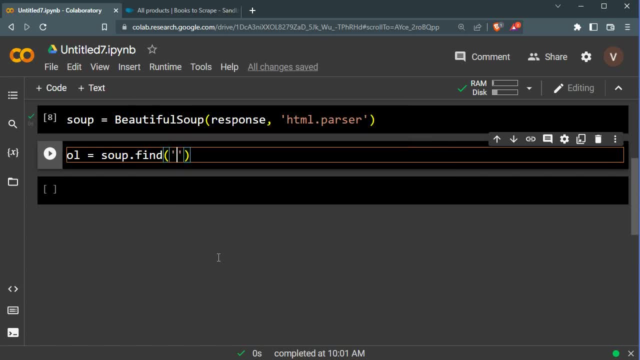 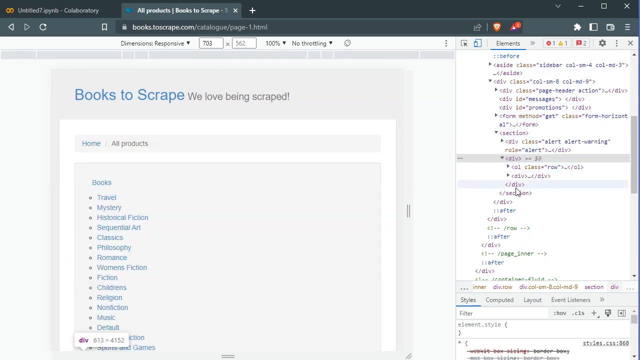 find method. the first instances are instance of order list inside quotes, double or or single quotes. so it means it's going to go inside the soup that we just saw or the HTML and find the first order list that is finds. so you can see this is the first, anyways, among all of them. this is so it will grab this find. 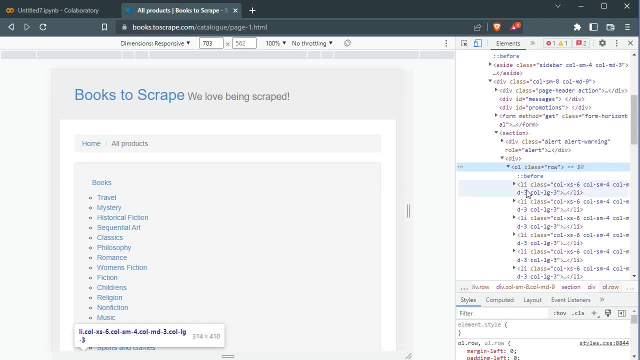 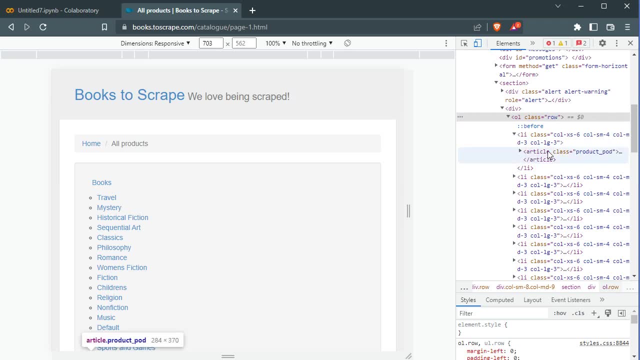 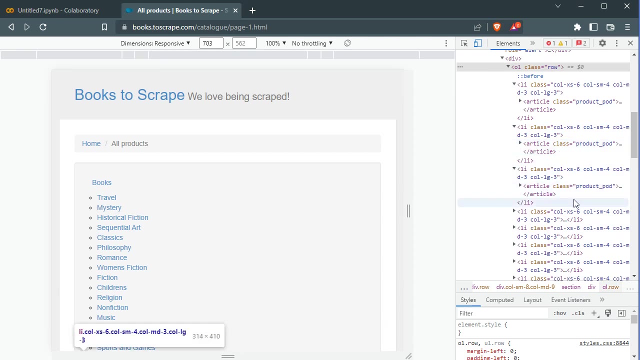 this. okay, now that we have saved this inside OL variable, we are going to loop. sorry, find all the articles now. all the articles, because you can see there are all articles here and inside the articles you have the price and everything else. so we need to find all the articles now. so that is why I've got. 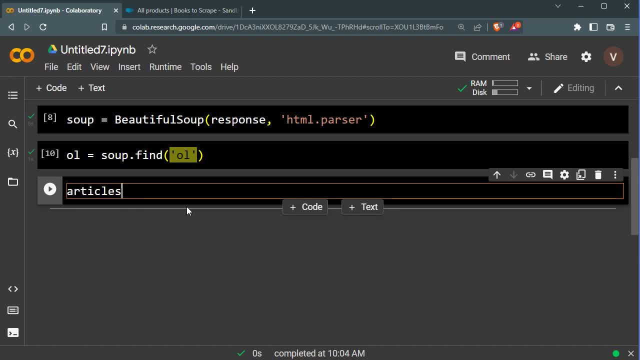 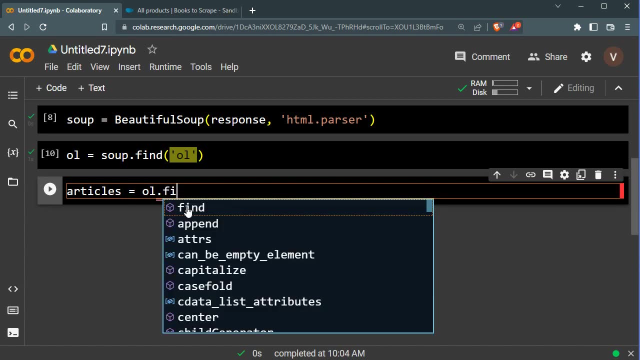 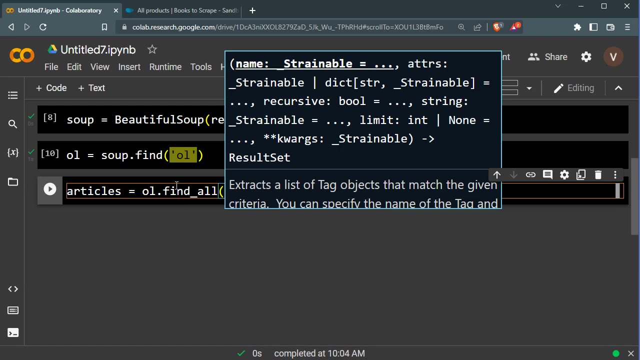 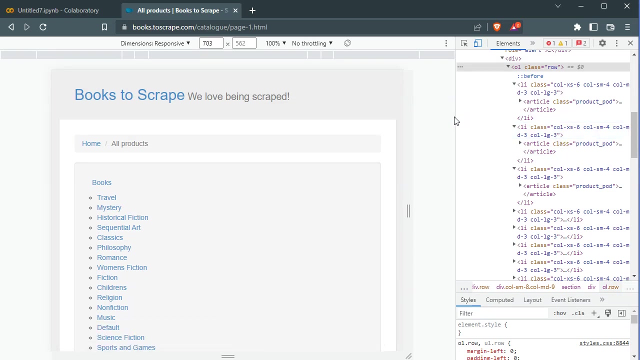 run this. I would have another variable. let's just call it articles equals, equals. now go inside the OL and find all underscore all. it will find all the instances of this article HTML tag and if you think there are some other article HTML tags as well and you want to be more specific, so what you can do, 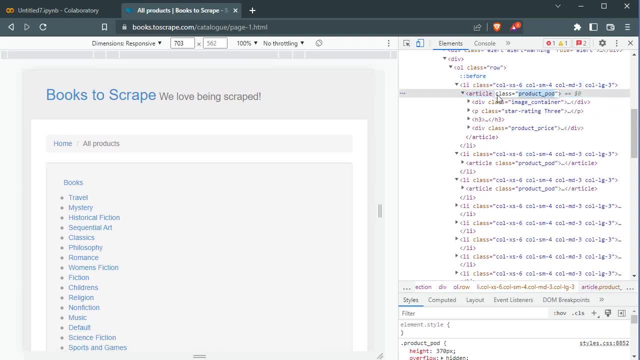 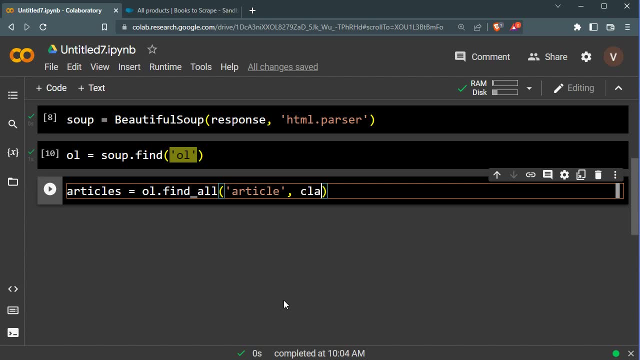 is. you can say: okay, I want to find the article tags with this class only. so we specify that here by comma class underscore, because if I just leave it at class, it's a Python class, but this is basically a CSS class or class underscore equals and the name of the. 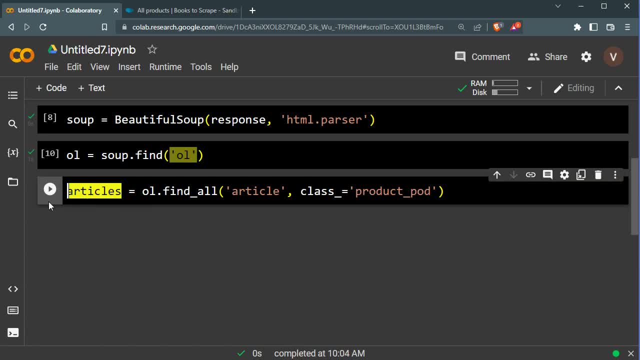 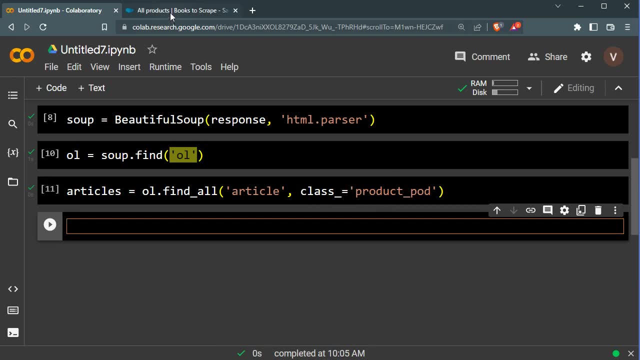 class. so now we have all the articles which are inside this OL. here let's run this, and now what shall we do? so we have a list of all these articles. I can print out the articles for you to see and you can see. these are all the articles like. 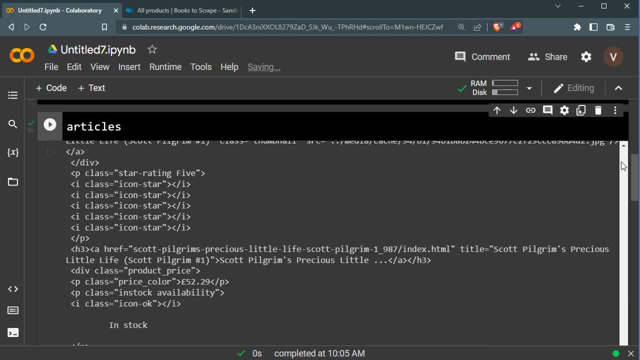 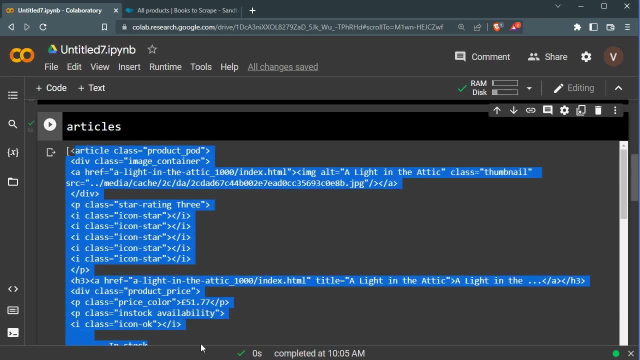 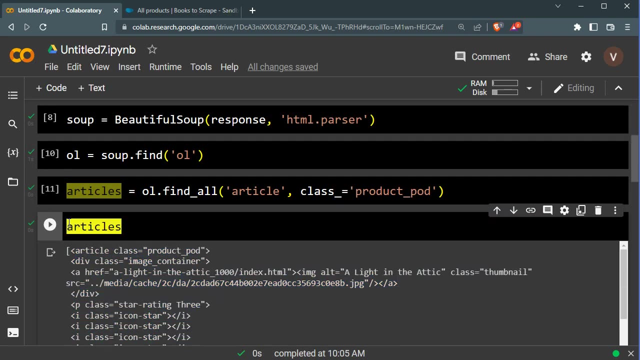 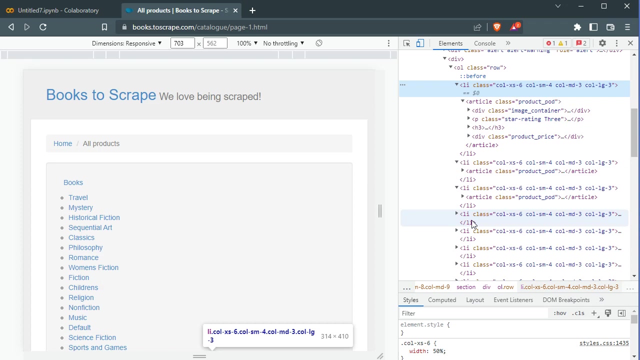 ends here, starts somewhere. in the very beginning you can see the list. it's a list which starts here with article and the article ends somewhere down here somewhere, and then another one starts. okay, so we are going to this time to loop through, to loop in all the articles and grab what we just talked about. the 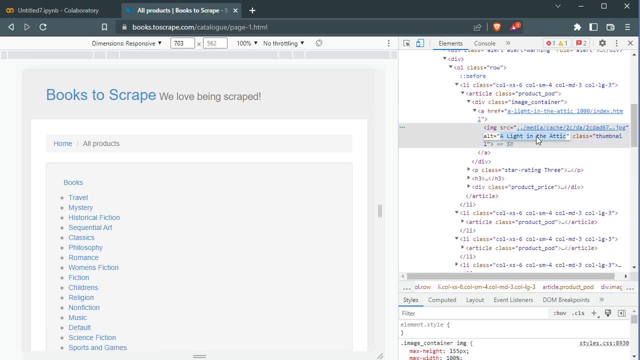 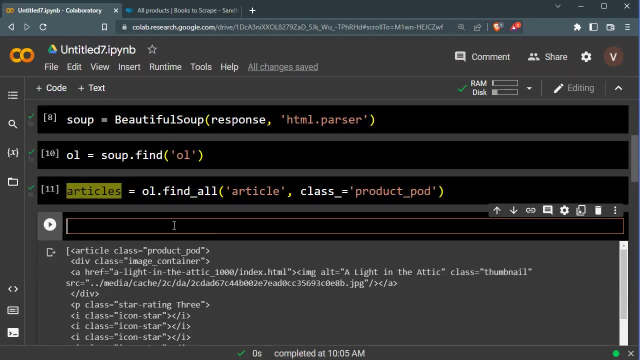 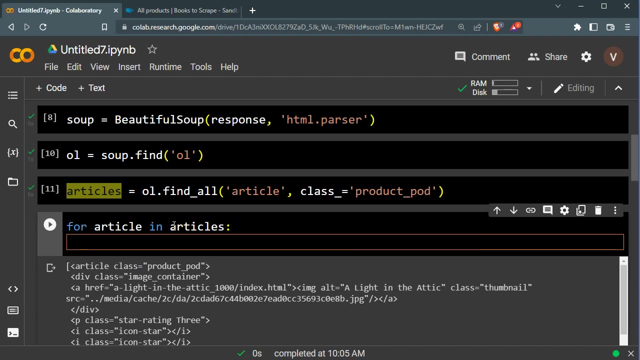 image, alt value, the star class and the price. so now let's say for article or I or whatever in articles, our list, the list that we just have here. so now let's say for article or I or whatever in articles, our list, the list that we just have here. 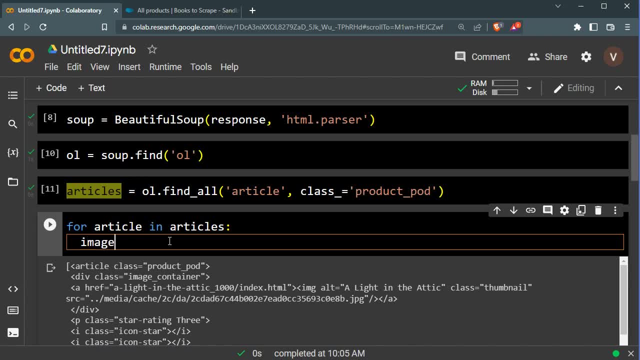 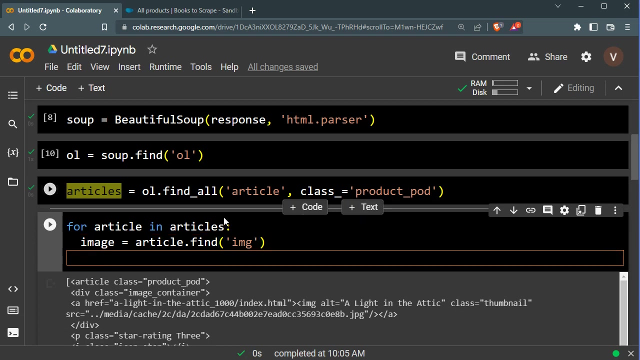 we need to do something. let's first grab the image. where is the image, the image? it inside the article, that individual article that we find. and let's say, find you should find the first. well, there's only one anyways: the image tag. get the image tag for us and save it inside image. now we need to get access. 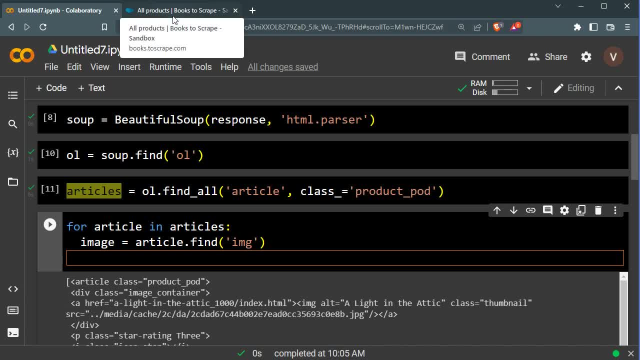 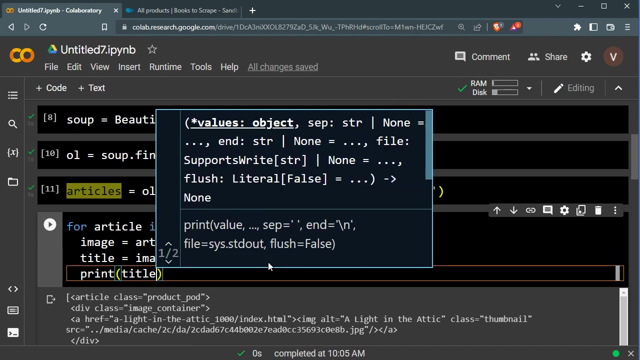 to the alt attribute, right? so I would say let's just call it: title equals image. that is the image that we just saw and attributes ATTRS stands for attributes of that image and what is the attribute? we're looking for, alt, and give us that title. so now, if I say print inside the for loop, if I say print title, let's. 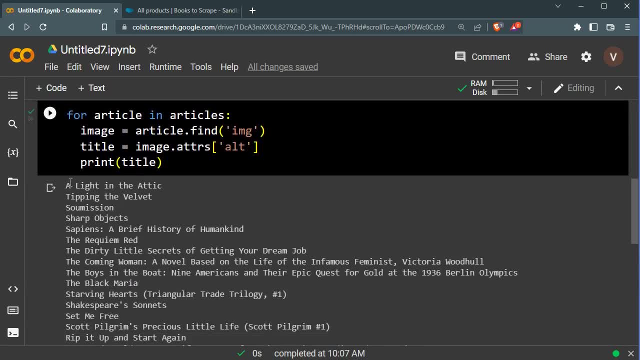 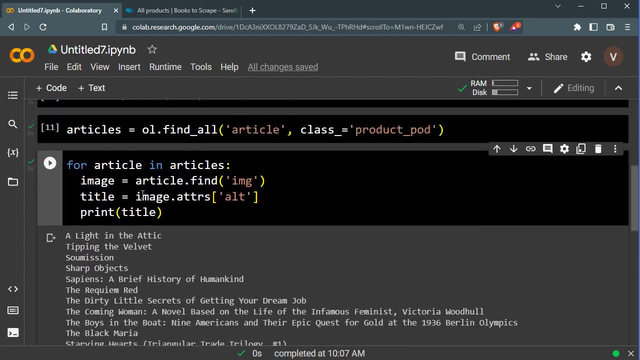 see what happens. you can see I have access to all the titles of the books on the first page, right. so that is what. how it happened. we found the image first and then we said, ok, now that we have the image, I want attributes: alt, ATTRS, alt and. 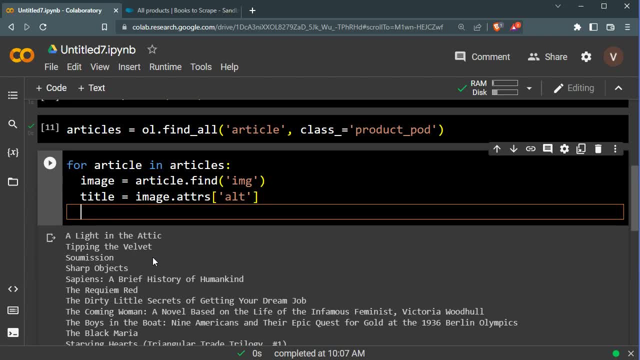 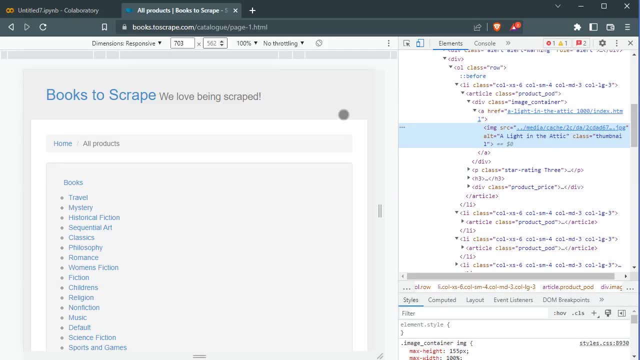 save it inside title. ok, now we have access to title. what about stars now? so let's say, star equals. where was the star? let's find it again. it was here, a P tag with a class of this right, and remember this is the the first P tag inside the article, so it's easy to. 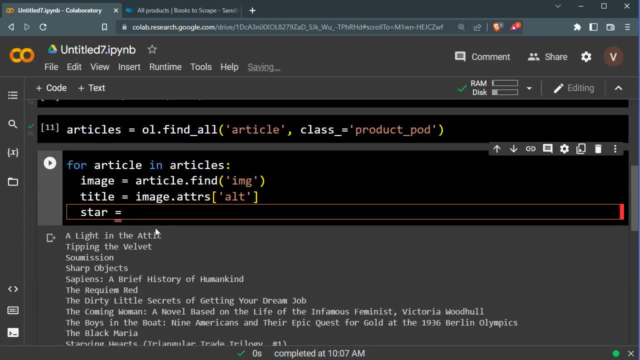 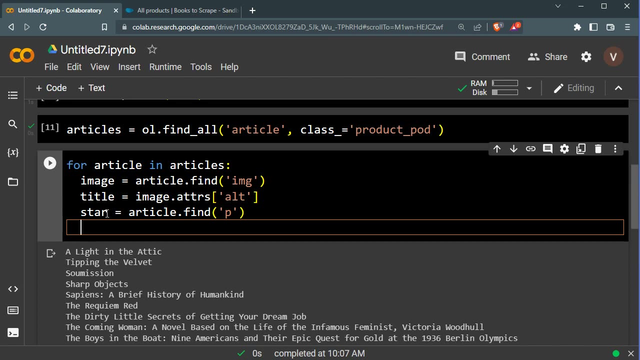 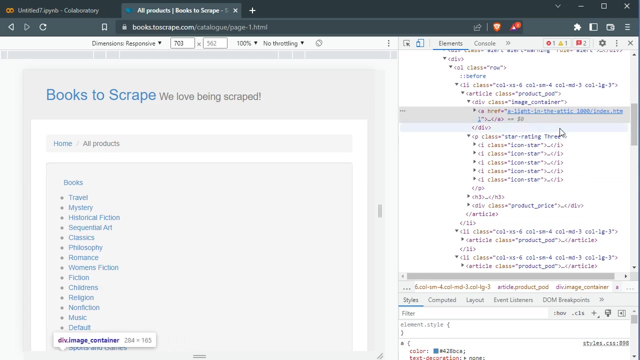 find now. so what we do is, I would say, star equals article dot find P. right, that is find a P tag. but there is an issue here. so if I print out this, you will see it. it prints out the whole thing here. I want the name of the class it has, I want to see which. 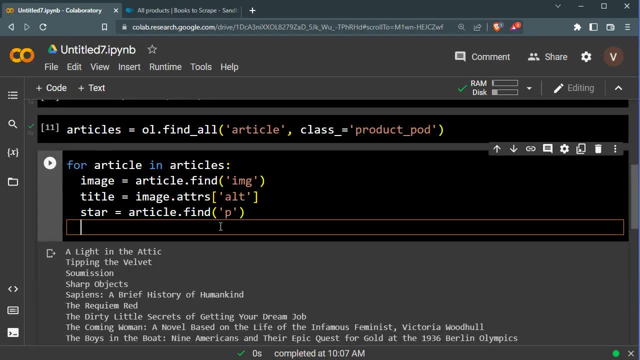 class name it has. so I would say again: star, equals. I'm going to redefine again equals star, which is the same star, and this time get me the class, because now it's more Patrician, because today I'm going to interati and Howling because I 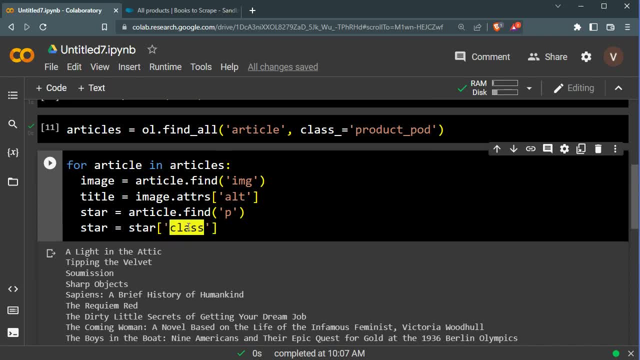 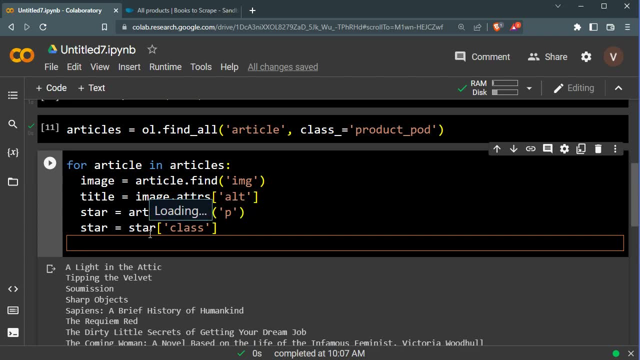 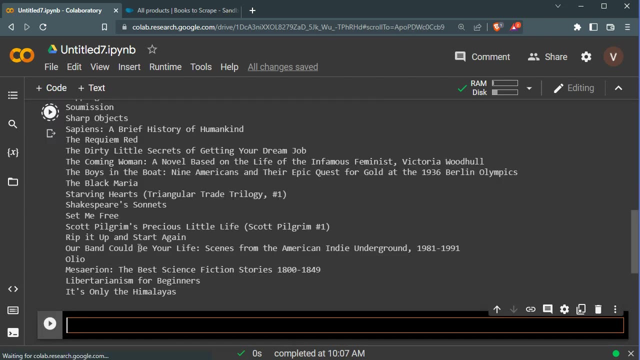 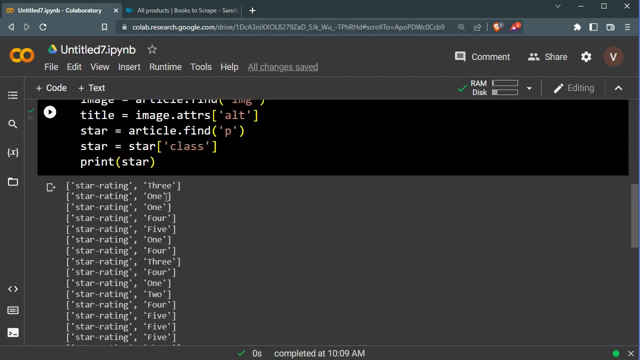 like a dictionary. so if we say class, it grabs the the name of the classes in a dictionary if they're more than one or whatever. so now if i print star, let's see what we get here now. so you can see now we have a list actually of these uh classes. so star rating, three star rating. 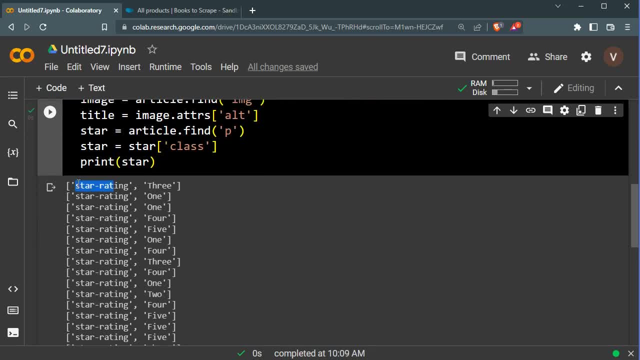 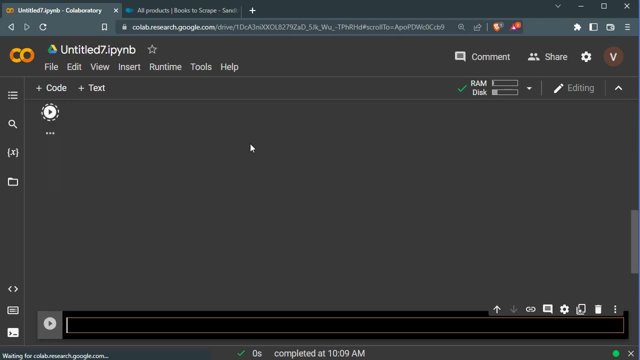 one, star rating one. but i don't need the word star rating, i just need the, the rating itself, which is three, one, one. so how do i access that? here i say: give me the index one which is this one, this is index zero, this index one. now i would only get the numbers. you can see a three, one, one. 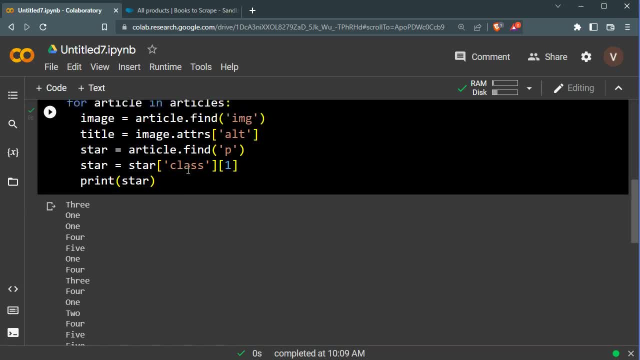 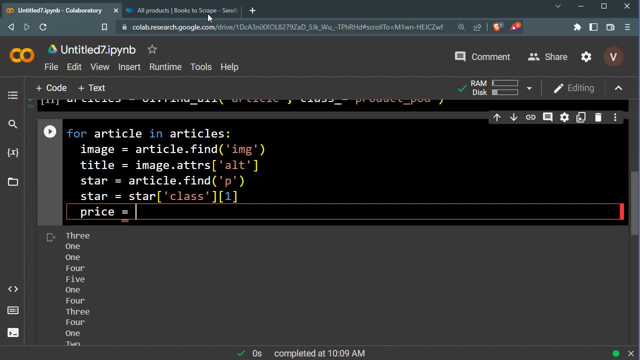 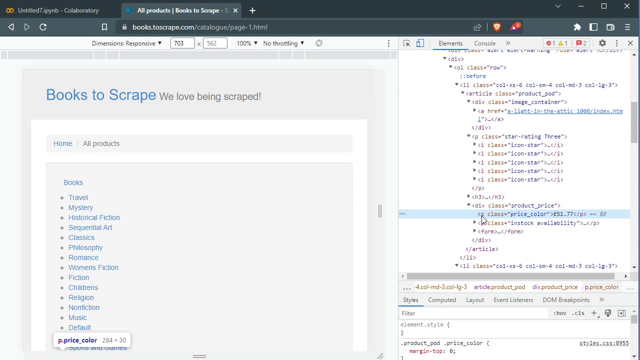 four. great, okay, so now we have also star. the price should be much easier, i guess. so price equals. where can we find the price under this tag here? so it's inside a paragraph tag with this class. you just need to zoom in and narrow down as much as possible to be more specific, 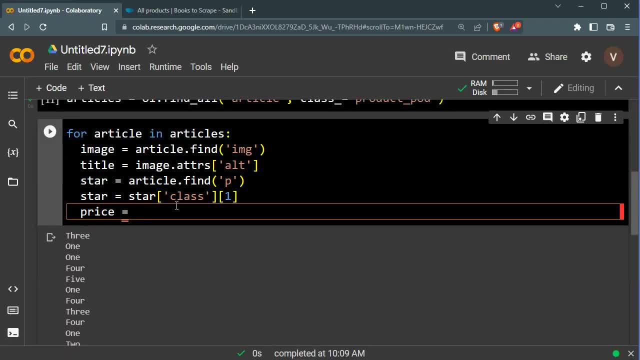 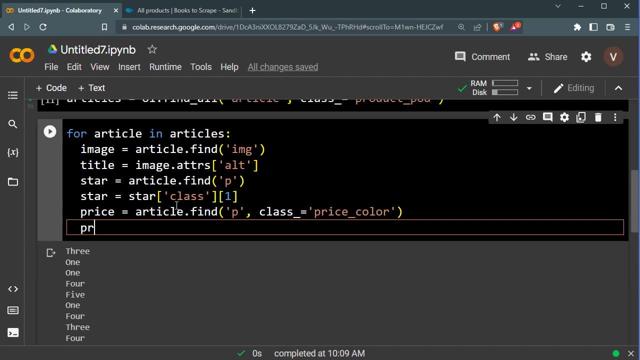 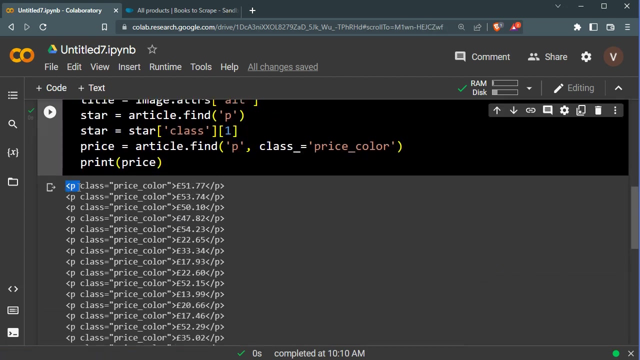 okay, so a p tag with this class name of price color is equal to article find is a p tag and the class name is equal to this right. but there is an issue. so if i print price now, you will see what happens. it prints out all the html tag p class and then price is here. i just need the text inside this. 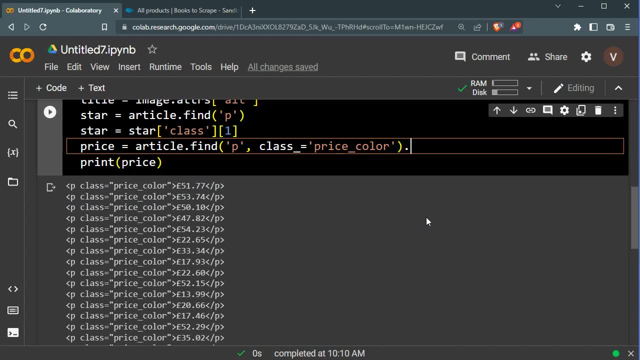 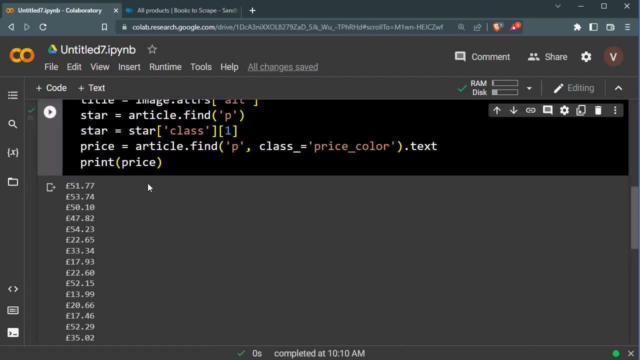 that's why at the end of this find i add dot text and now you see we have this. so if you're happy with this, then it's fine. but sometimes you might need to have numbers so that you add some stuff or arrange them in order, you know, from high to low or low to high. 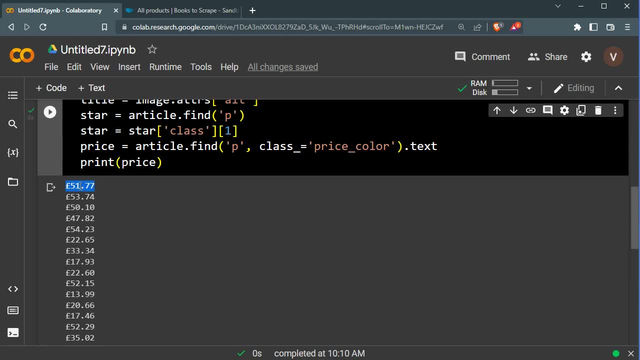 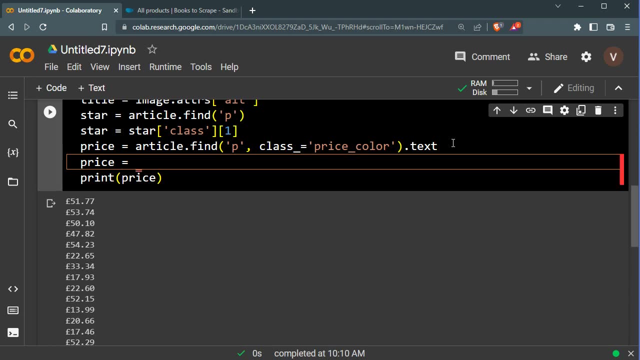 so, but this is string format. so what we need to do, let's just do something with it. so what i can do, i can say here, price is equal to: or yeah, let's just have it like this: it's cleaner price from index one up onwards. that is, this is the price, this. 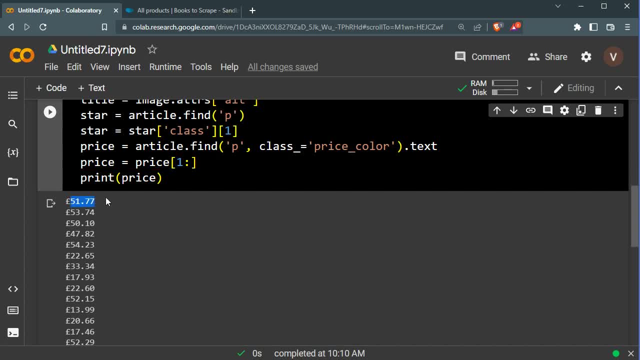 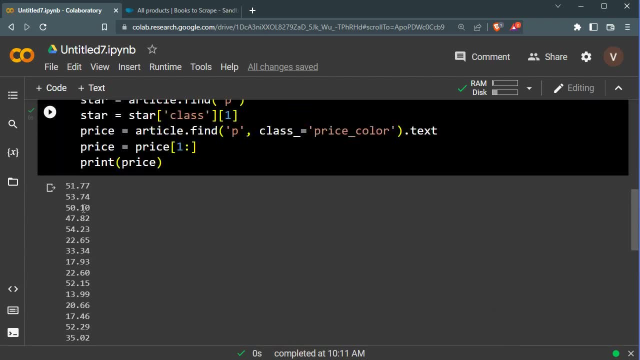 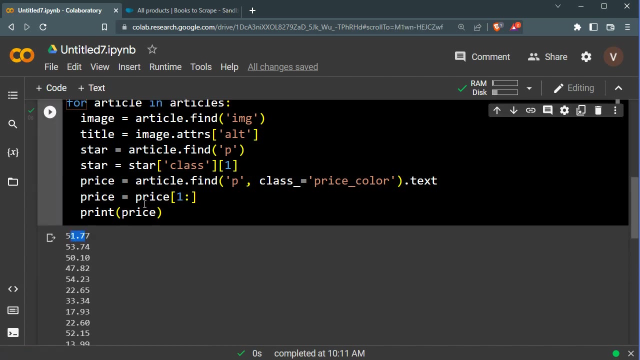 index zero. i want only from index one onwards. i want this part, only this part, only so now i would get rid of this symbol, the great pound, great british pound symbol. okay, but still, this is a string. so what i can do, i can turn all this into a float. 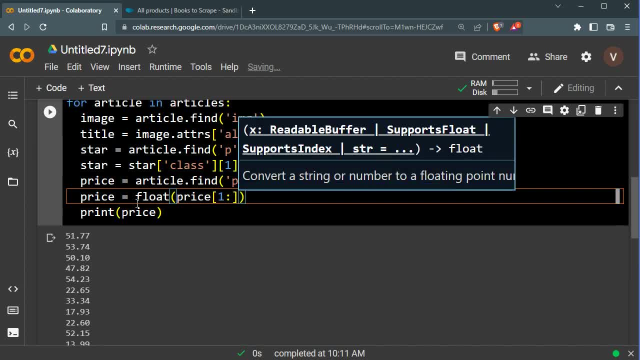 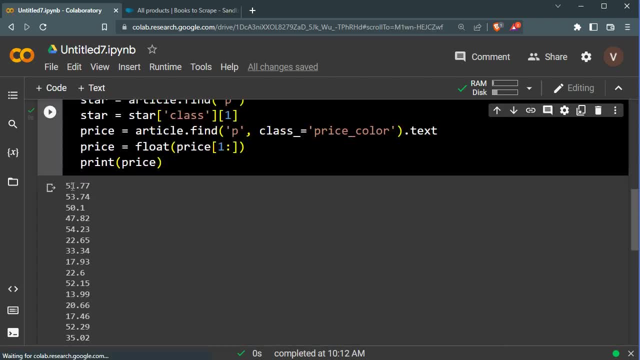 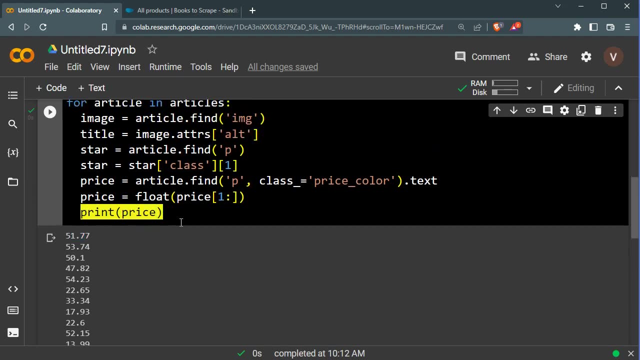 with. i mean, float is a number with decimals, right, so i can wrap it like this: and now it looks the same, obviously, but now it's a number that you can add to or subtract something. okay, we have now our uh, title, stars and price, so let's put them all um inside a variable, maybe. 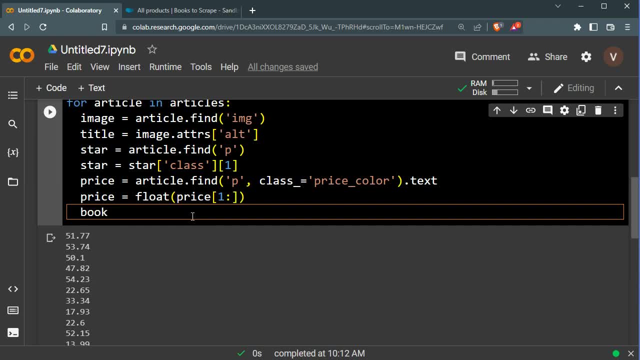 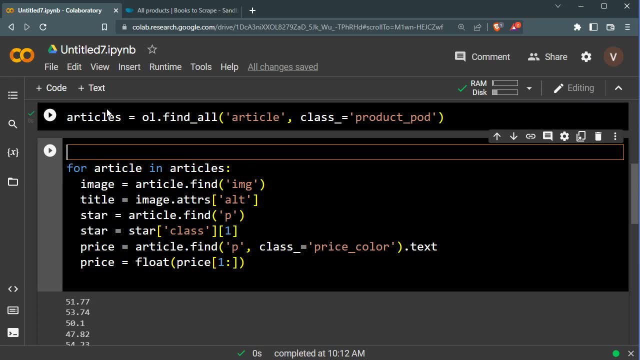 so we can say: i don't know book. well, actually, let's do something else. let's define a list of books here. so i would say: books equals an empty list, and i'm going to add all this information to this. so i would say, uh, books dot append. so we're going to add this books to this empty list. 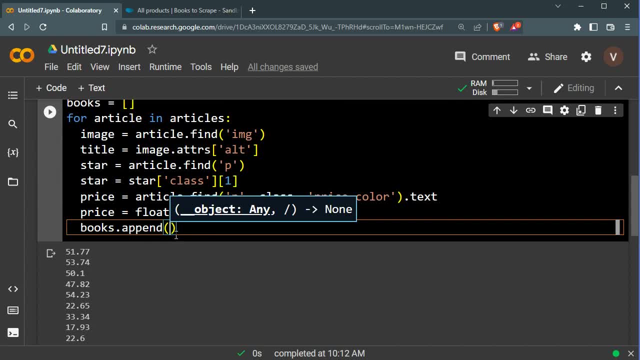 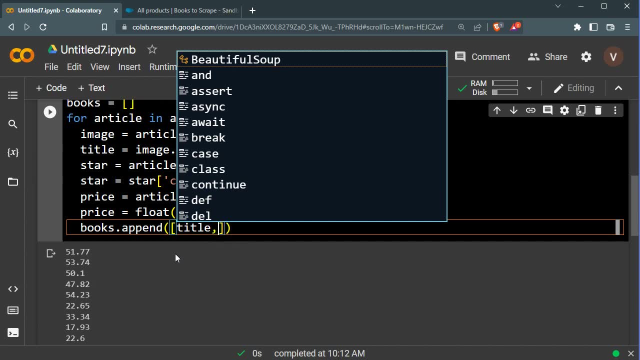 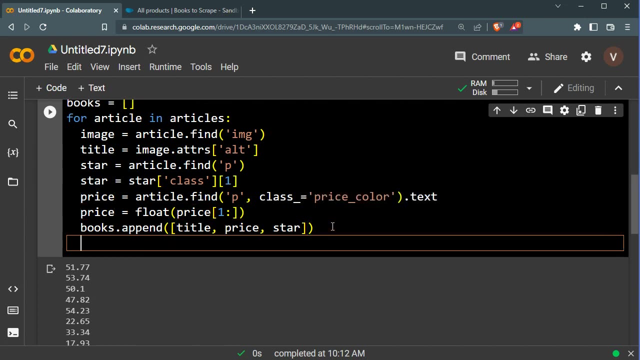 the uh, title, star and price right. so i would say i would say: title, star and price right. so i would would put them again inside another list, so that would be title, then maybe price first and then star, and now I can print books down here and you will see, it's a. 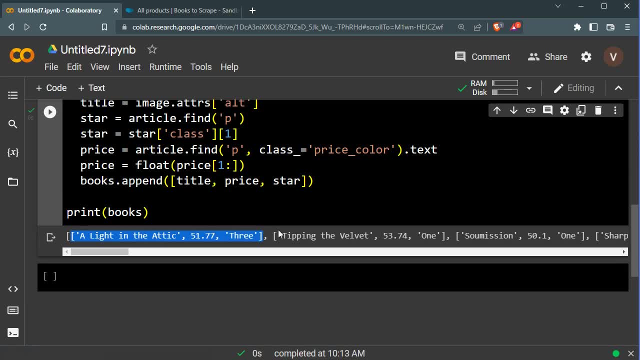 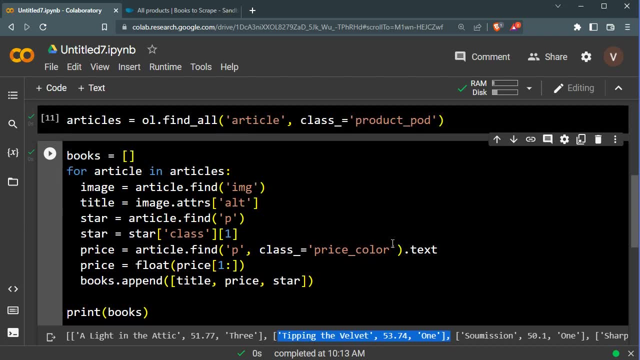 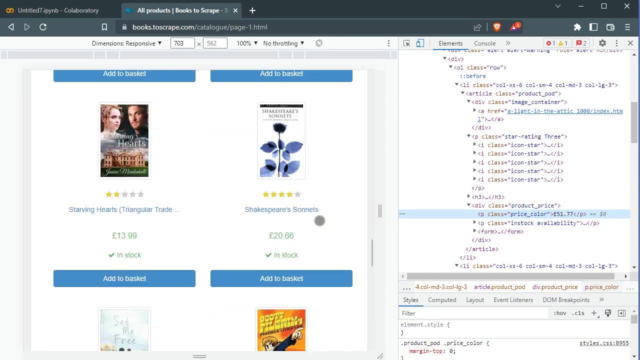 list of lists. you can see this is the first book, for example, this is second, third and others okay. so so far so good. but what we have been doing is only for one page. that is the first page. what about page 1 to 50? all of them? well, the 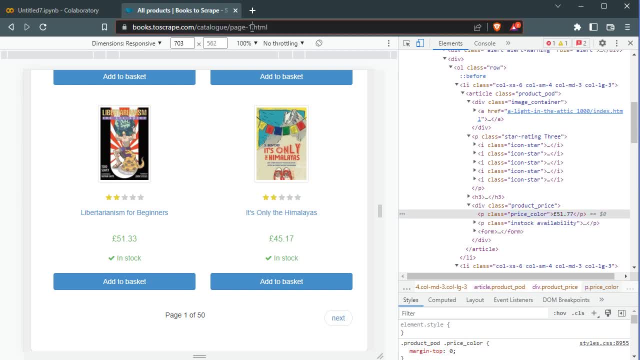 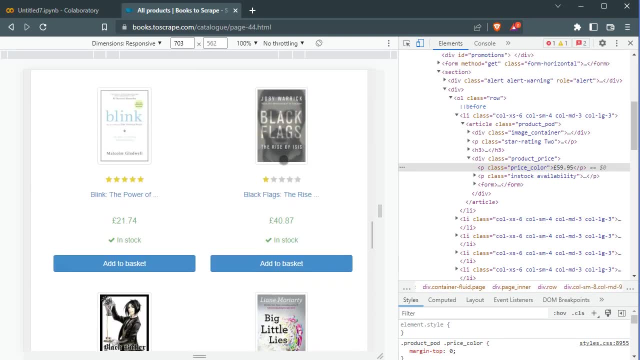 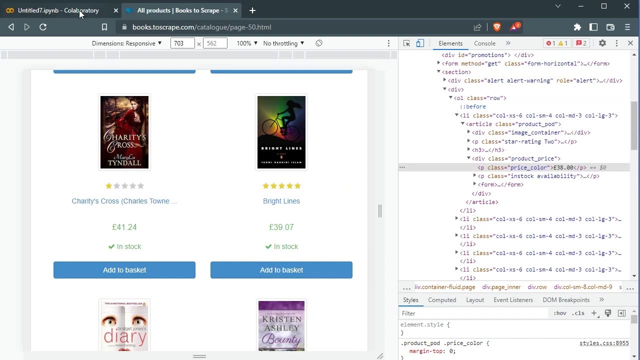 trick is, if you see here we have page dash 1, if I change it to, for example, I don't know- 44, then it will show me this one right. so I can go up to page 11, 50, right, like this. so I just need to update this number. so what I can do is 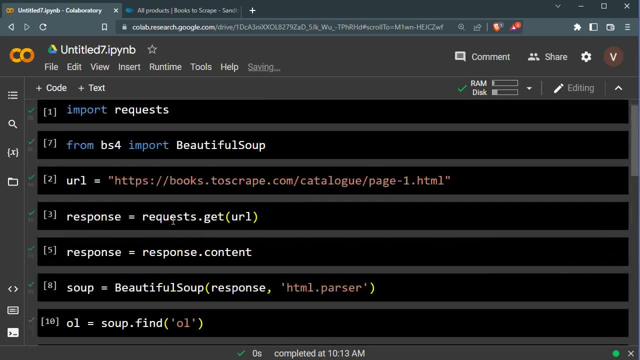 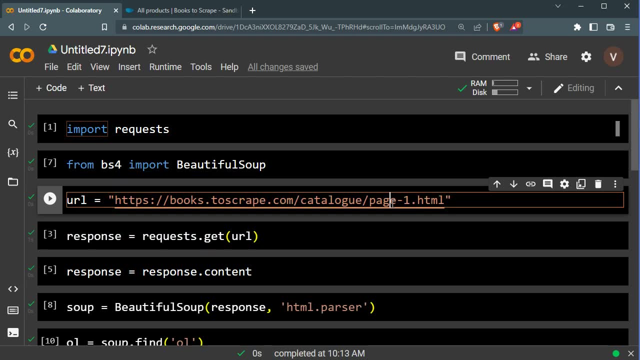 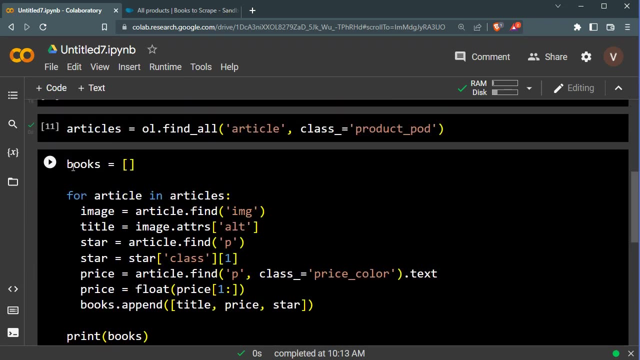 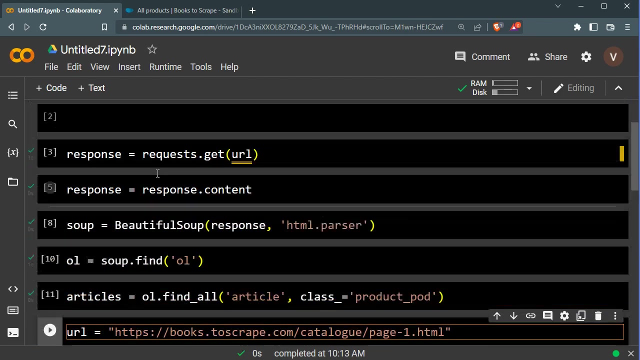 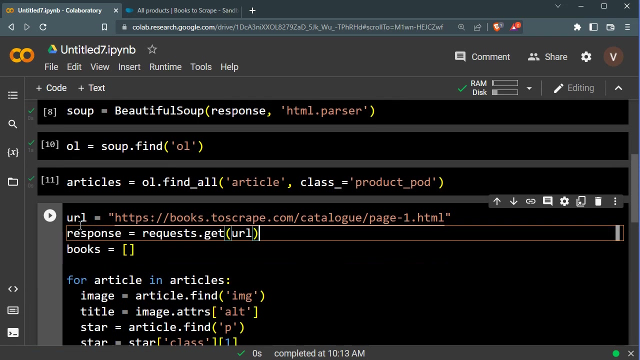 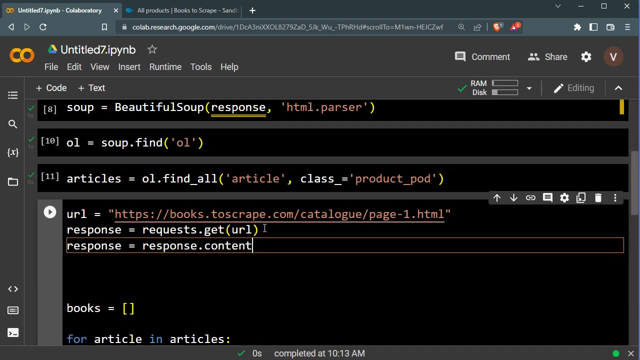 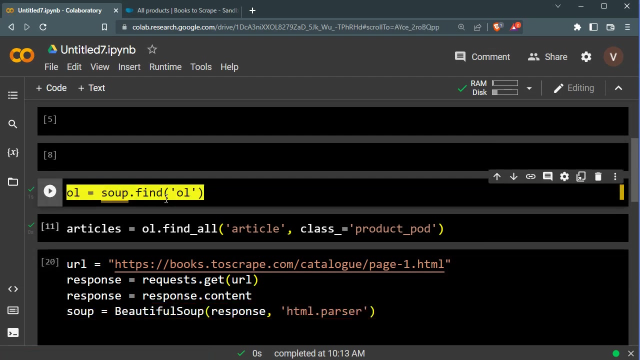 like here. I can say instead of this: where was that, this URL which says like number one? only let me grab this. I want to put everything in one cell list, like here, and also this one as well: here and the content here. what else? the soup that we made here, the order list we grabbed here and the articles inside the 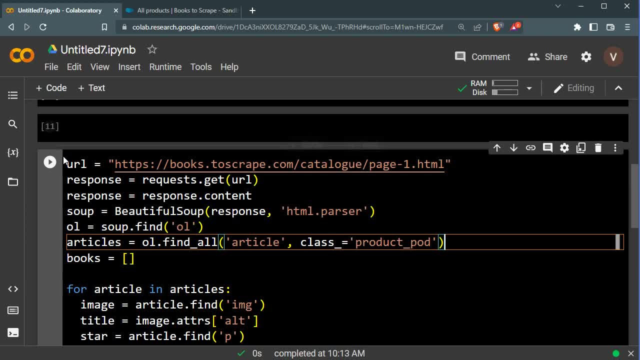 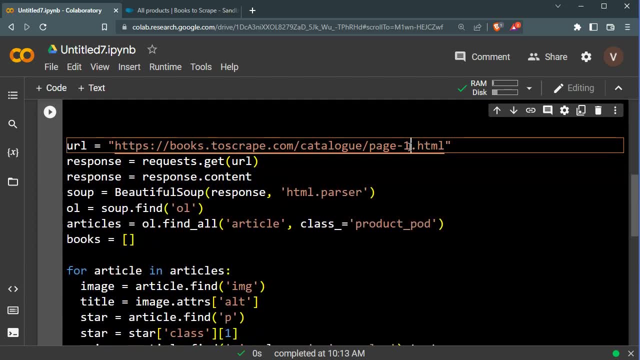 order list we grab here. okay, so what we need to do is to say: now you did this process for only page one, then do the same process for page two or page three, page four. that is why we are going to update this and put it inside a for loop. 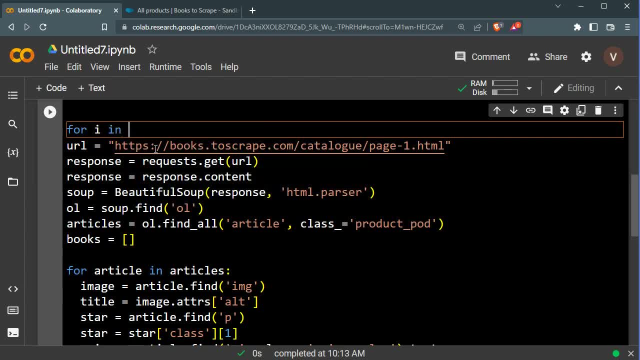 I would say, for I in and we're going to give it a range of one to 51, that is up to 51, but not including 51. there is one up to 50 and including 50, because we know it's 50 pages, right. so from one to page 50 do. 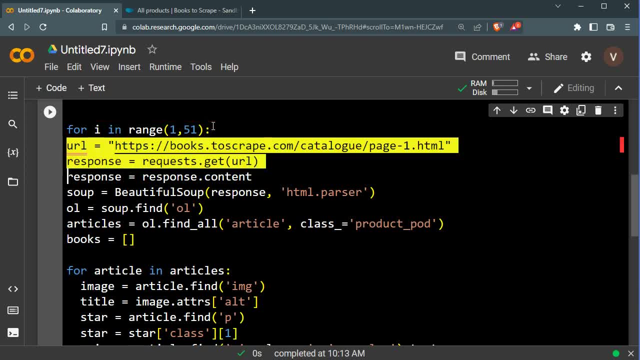 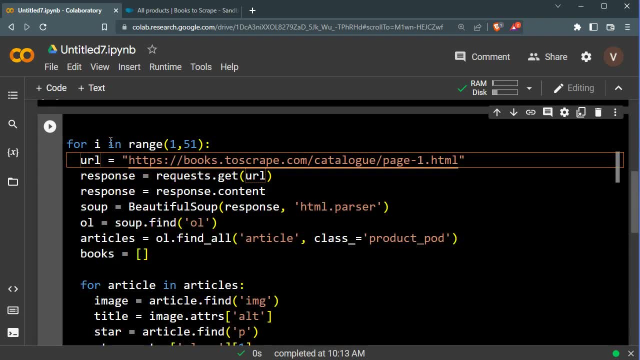 something to what. so let's put everything a tab and we've indented under this. now what is a? I is going to be one, then runs all of it, and then I will be two and runs all of it. so instead of this page one, now we can put I, and at the beginning let's put an F string. so now, 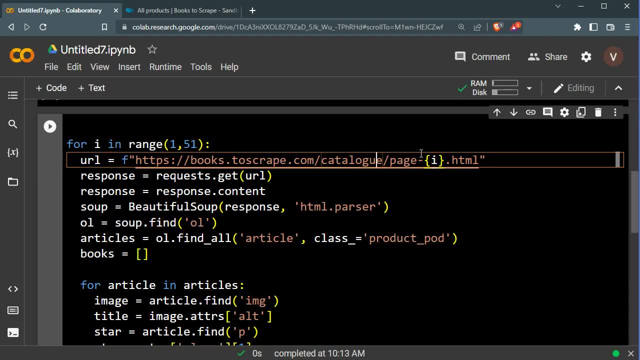 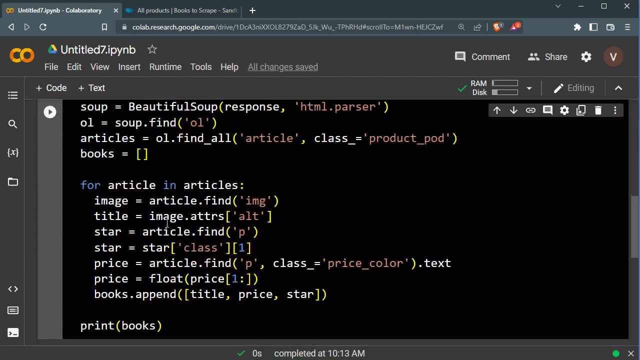 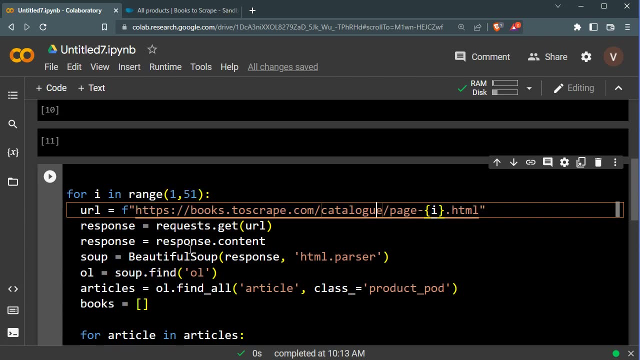 it is a variable. so the first time I will be one, page one, and then we're going to send a request to page one and do all that here. then, when it's done, I will be two, so it would be page two. so it will go all the way. 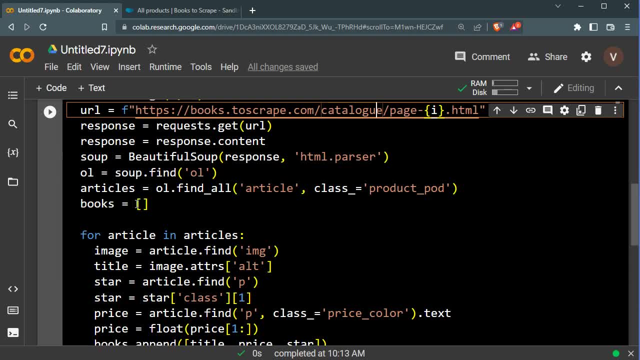 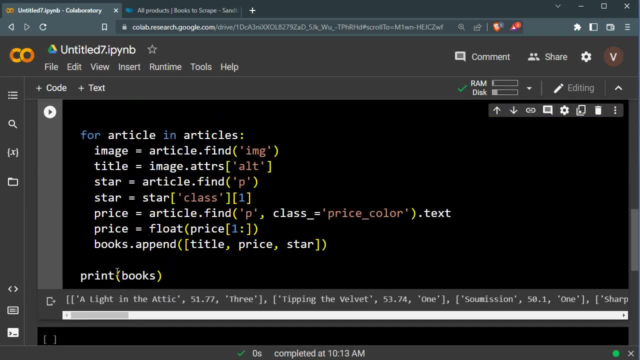 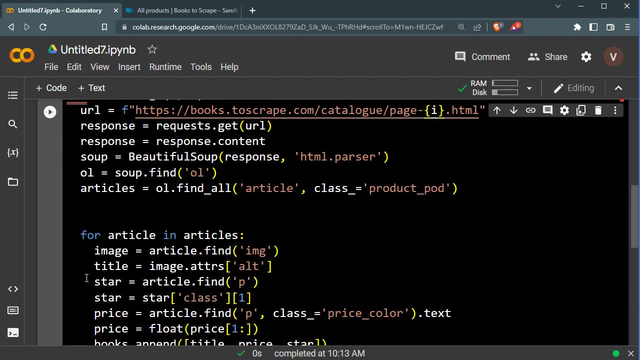 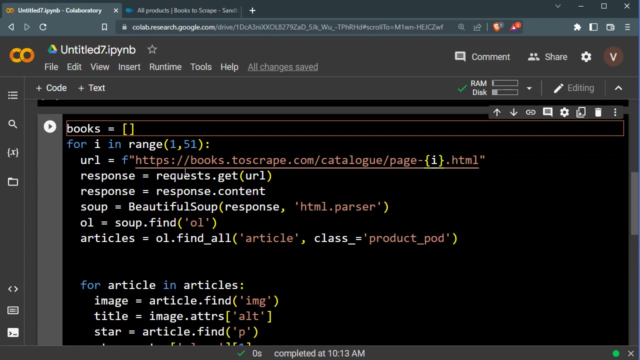 up to page 50, but then we don't need to have this books here inside the for loop, and also this one. we don't need this either. I will tell you why now. okay, so this will basically be the indentation. okay, so this is basically the same it. 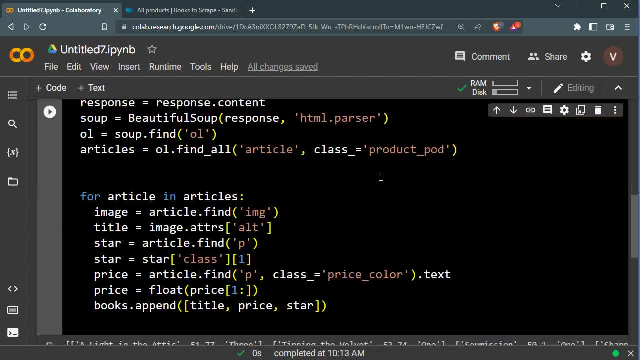 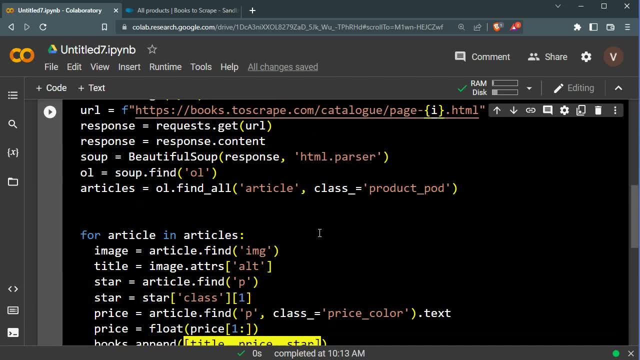 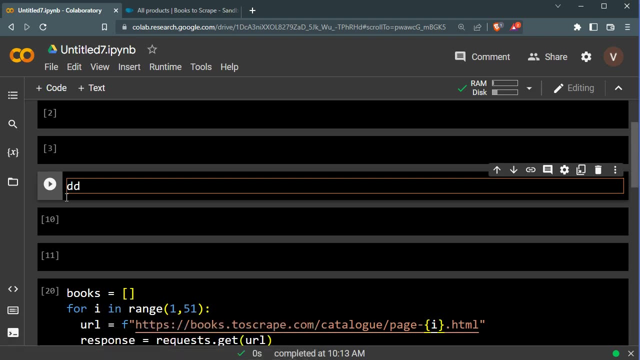 just goes over the process for 50 pages and does that. that saves everything inside a list. but what about P and CSV file? how do I export it? very good question, okay. so here we have all these oops, yeah, so let me get rid of these now. 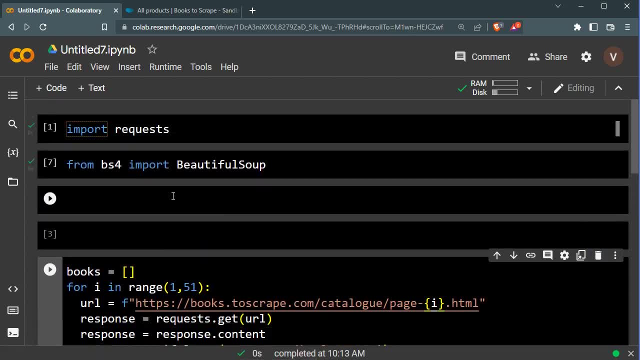 and so here, let's import pandas as a PD, and we're going to use a pandas library to export this information to a CSV file. if you're using your machine, you have to install it: pip install pandas or pip install beautiful soup or pip install requests. don't forget that. okay, now that we have access to pandas, we 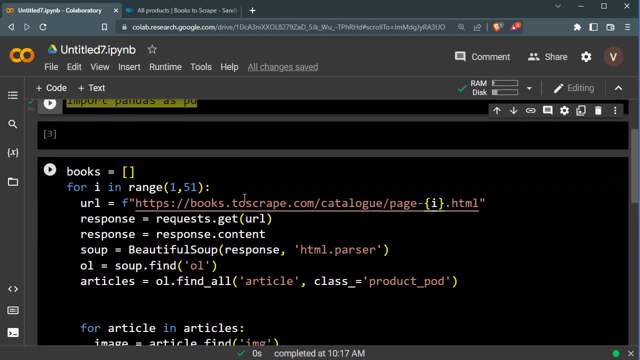 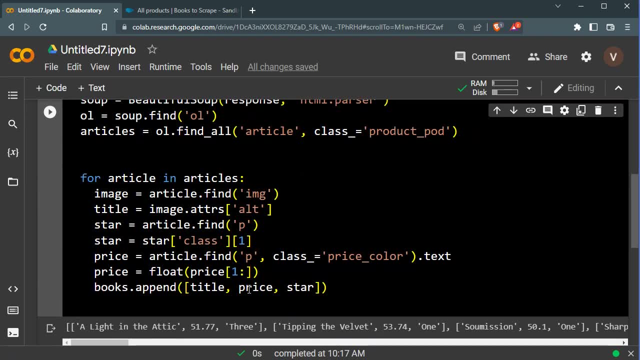 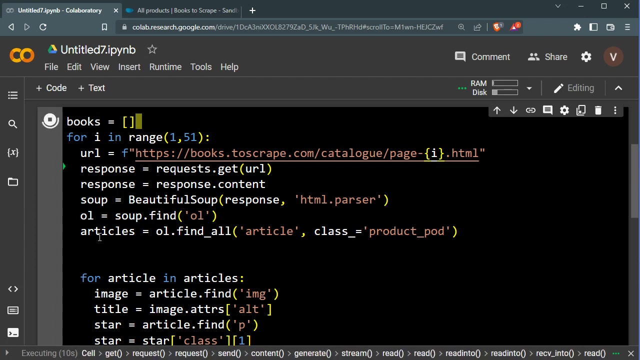 around this. I guess, yes, they would check. okay, now I can say, now that we have the books right, which is full of all of these books. so let me run this so that everything from all these 50 pages is saved inside books. so you see, it's running it and it's gonna take some time because it's 50 pages, obviously. so 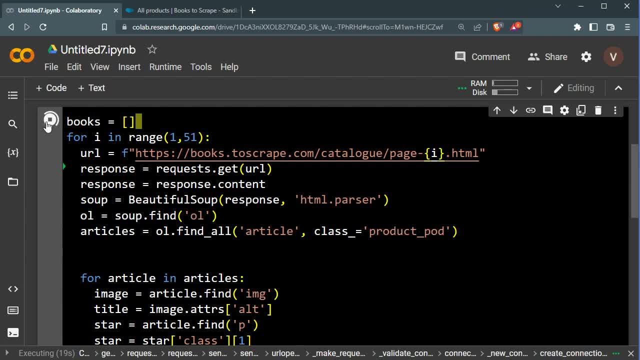 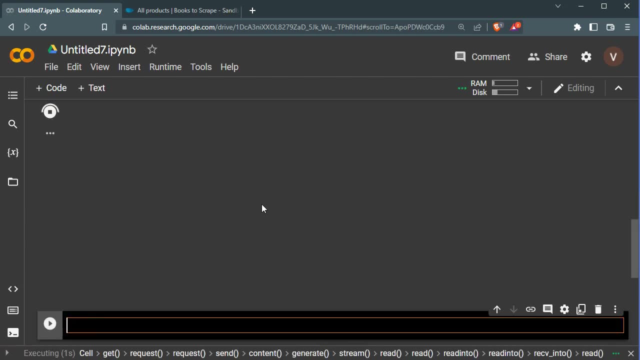 or I can stop it and just go for- I don't know- four pages or five pages. so yeah, I'm going to stop. this is too much. so what I will do is just say, okay, for five pages, for example, let's do it for five pages, and it should be faster now. 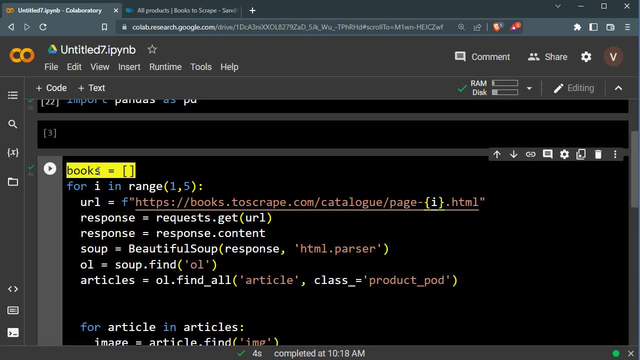 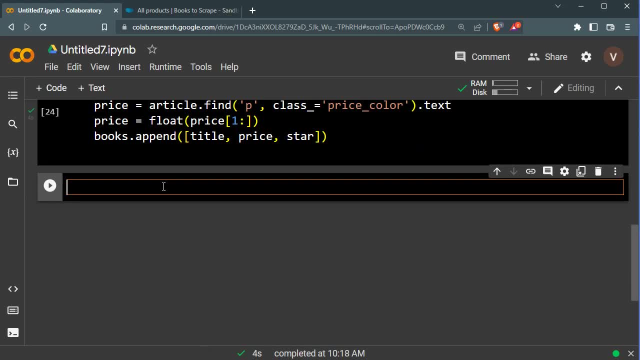 yes, it's done and everything is inside this list of books. so for pandas: pandas works like this. pandas needs to have access to data frames, for instance, and data frames are basically like tables, like CSV. spreadsheet got tables, so we need- we need to create one data frame like DF. 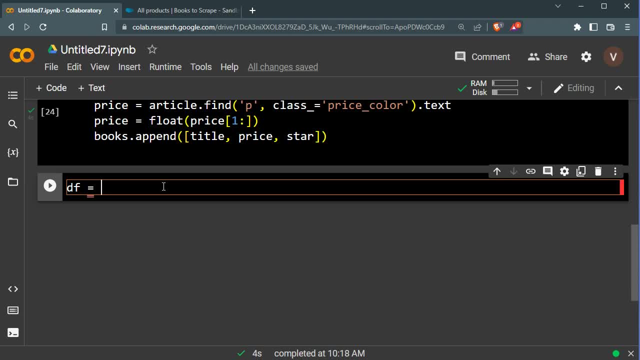 you can call it whatever equals, and we use the PD, which is pandas, as we imported dot data frame method. so we are going to turn something into a pandas data frame. and what is? it is going to be the books that we have now. I remember the books. this is a list of lists, right, and it doesn't have any columns at the 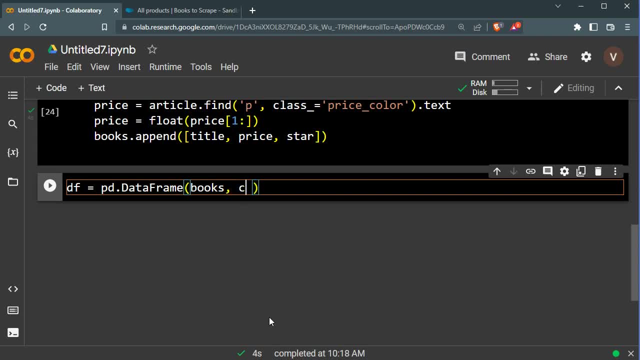 moment, because it's just like list of lists, so we can give it some column names. so columns equals another list, and the first one should be maybe title- I think it was title in the first. the second was price- yes, price here. so these are going to be a title, price and star rating. so these 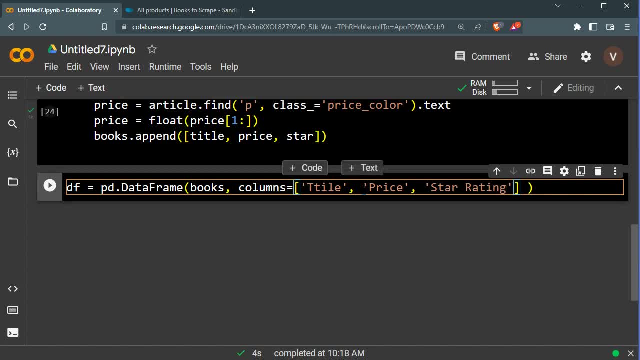 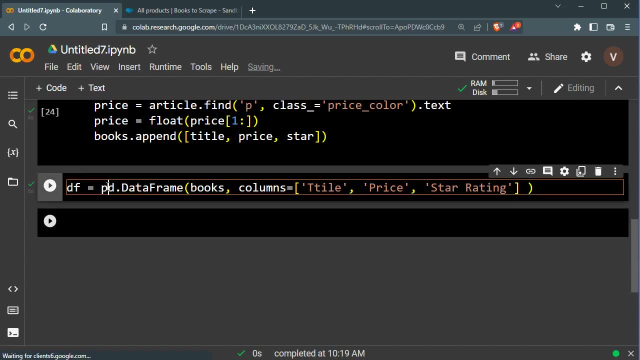 are going to be the columns for these lists and I'm going to shift, enter, run this, now we have access. now that I have access with this, I can turn it into a CSV file. so easy. I need just say DF, dot to oops, to underscore CSV and give it a. 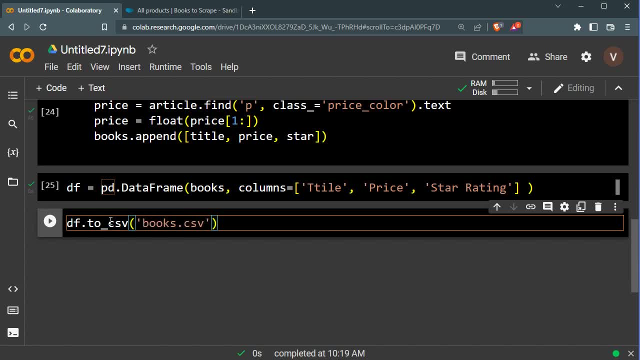 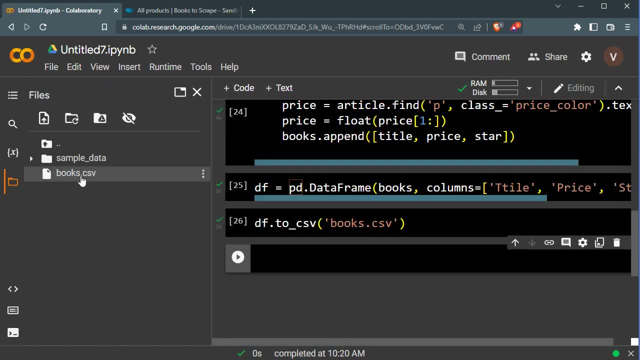 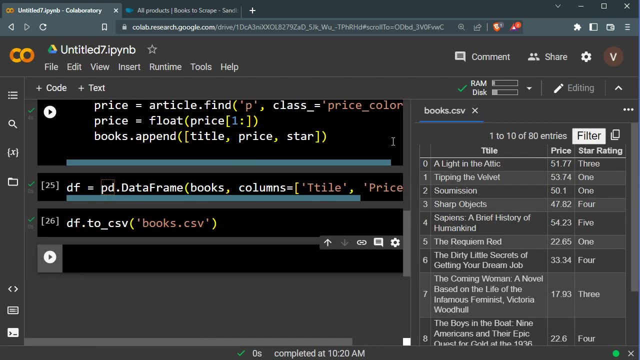 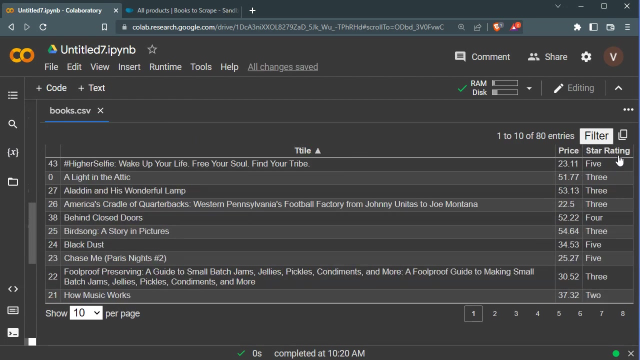 name, like books dot, CSV, for example, and shift, enter. and where does it go? well, it goes here and you can see, I have it. I can download it if I want to, or I can also display it right here. let's see what we have and you can see. we have this title, price and star rating.